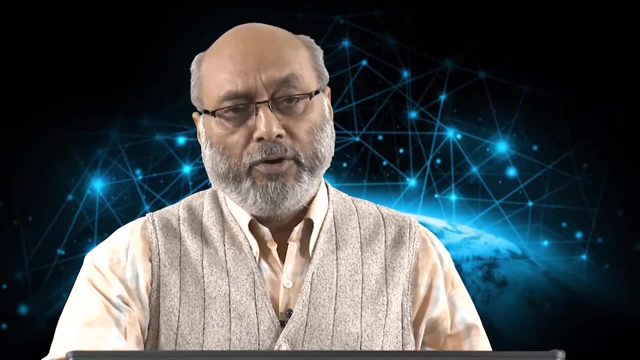 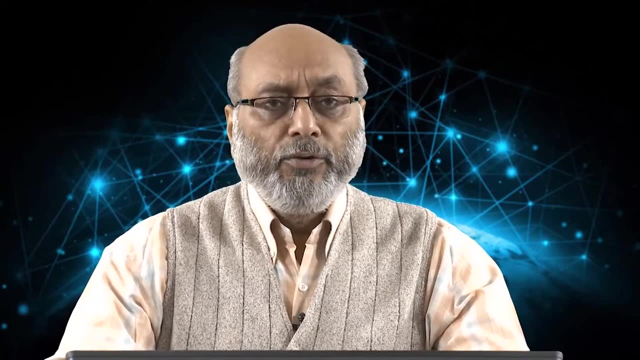 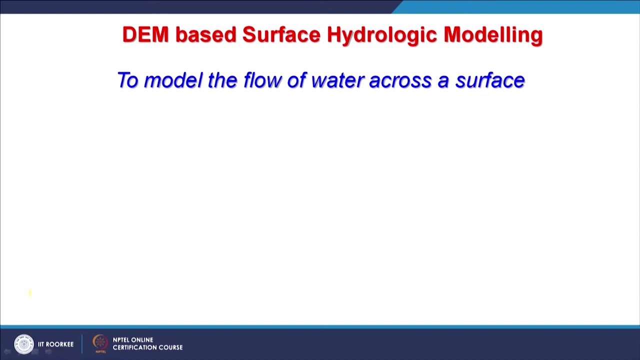 we can derive from Surface Hydraulic Modeling. So we will discuss in 2 parts. So let us start Now. as you know that whenever we say word modeling we mean to say that we mean to say model. Here 2 models: One is the digital elevation model and then Surface Hydraulic. 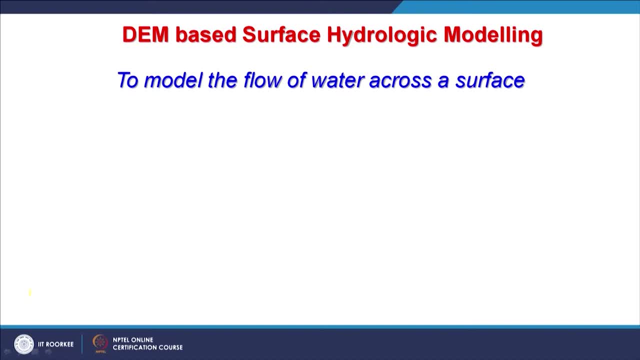 Modeling. So model means basically here the Surface Hydraulic Modeling, that to model the flow of water across a surface And surface here is digital elevation model. So we are using one model to model the water flow over the surface And specifically I have used 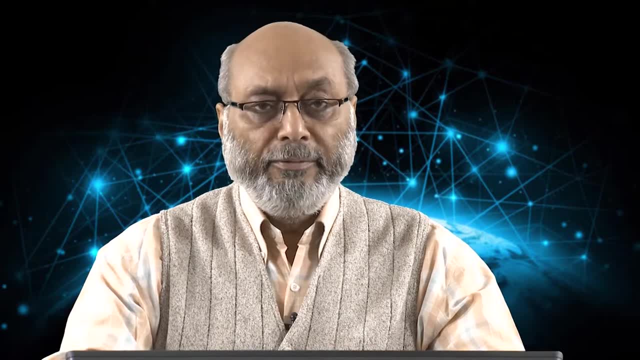 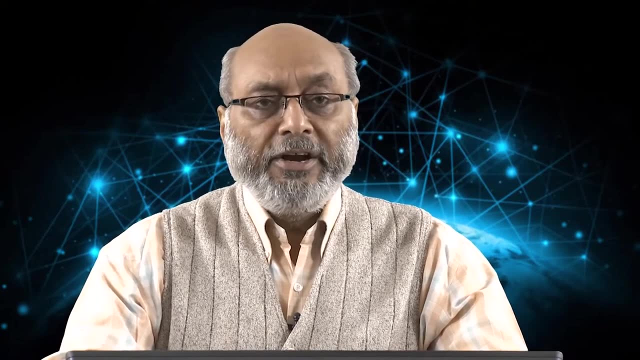 this term over the surface. So this is important, which we will cover in the next lecture. So this is important, which we will come later in the discussion, why I mentioned over the surface Now, as we know that the shape and characteristics of the earth s surface is useful in many fields. 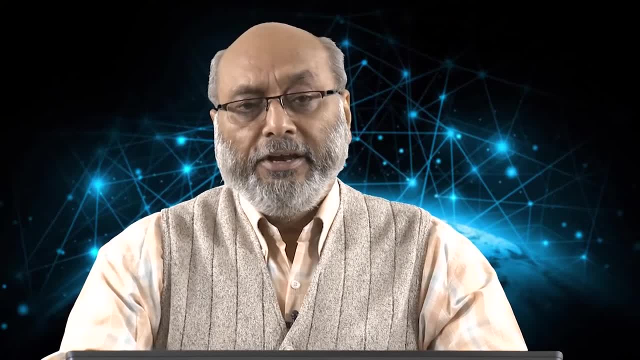 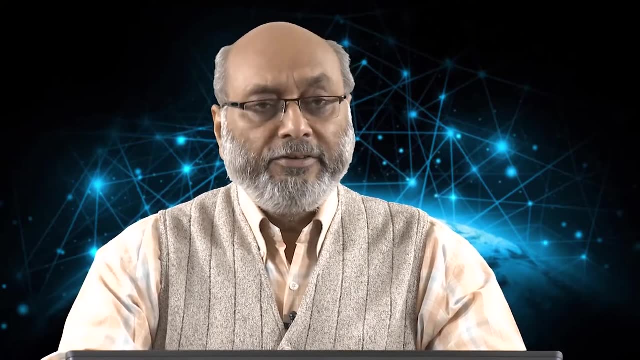 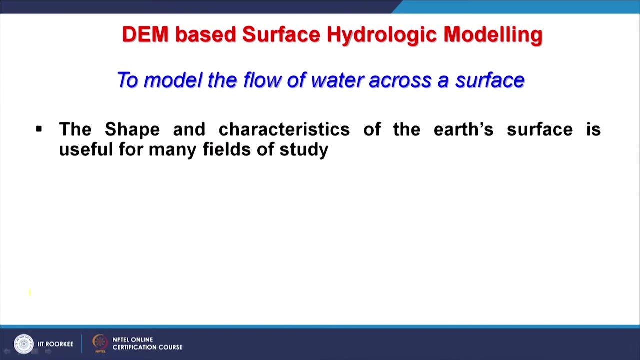 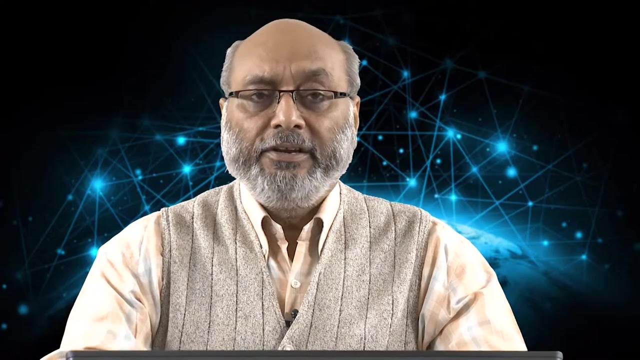 of study, especially like in civil engineering, in earth sciences, in hydrology, in geography also and nowadays in environmental studies also. So this shape and characteristics of the surface, And what is the model or what is the data which can represent the characteristics That? 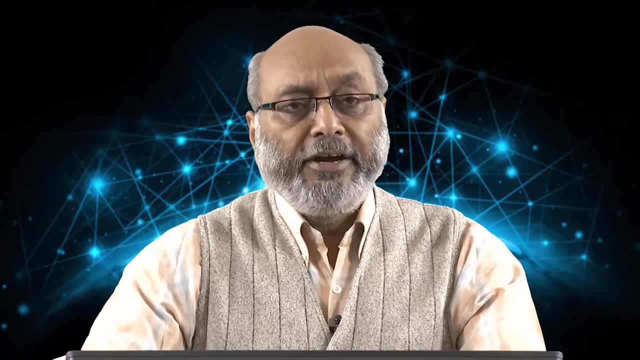 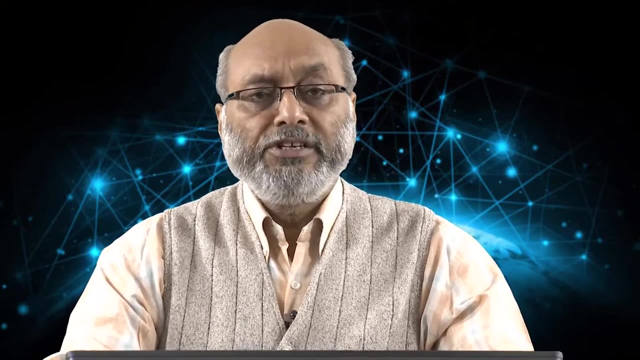 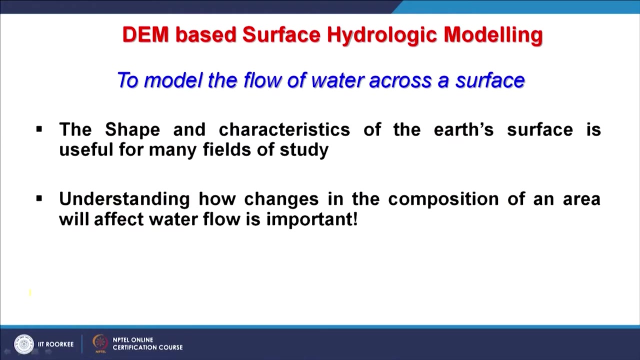 is the digital elevation model, And this understanding about the surface characteristics will also allow us to see how changes in composition of an area are taking place or will take place in future, And how water, when it flows over the surface, it creates different features or boundaries, like watershed, boundary and other thing which. 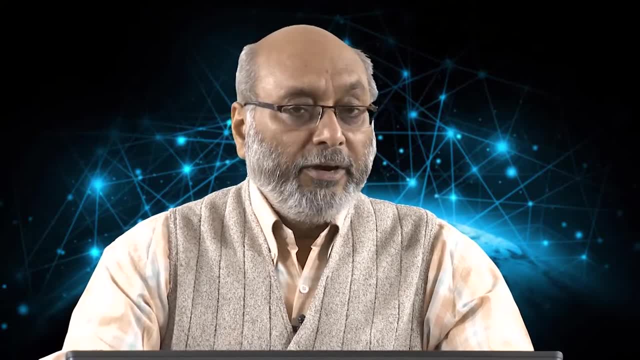 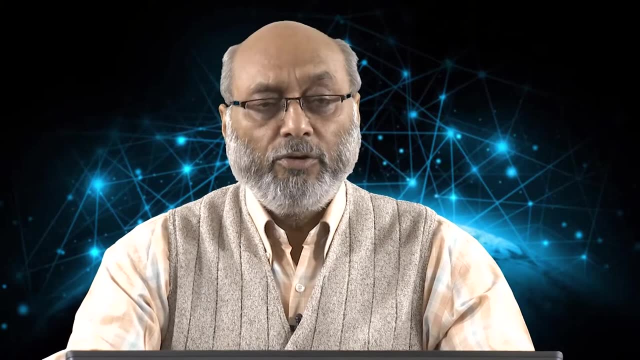 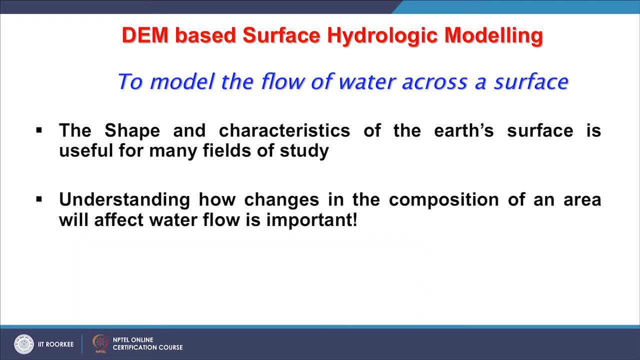 is, of course, a topographic boundary as well, But water flow- this plays a very-2 important role. Drainage network is also developed because of water flow on the surface, So we can try and what we will have through this surface. 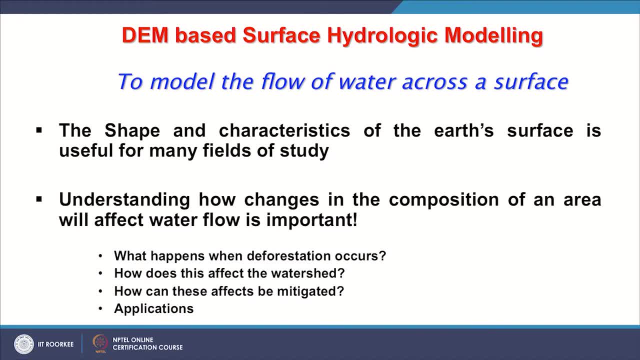 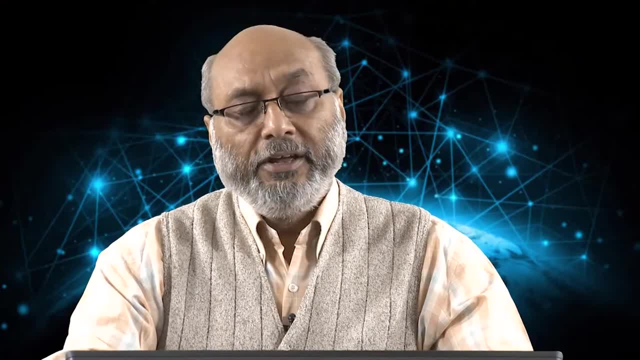 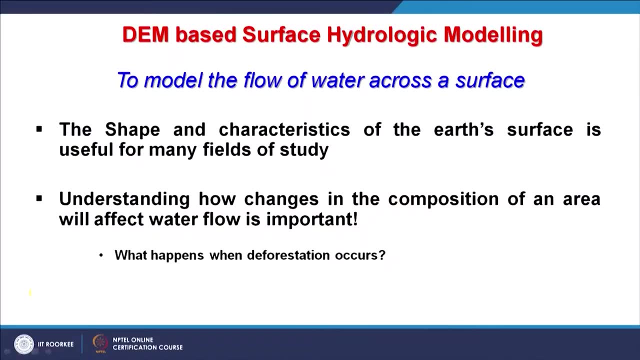 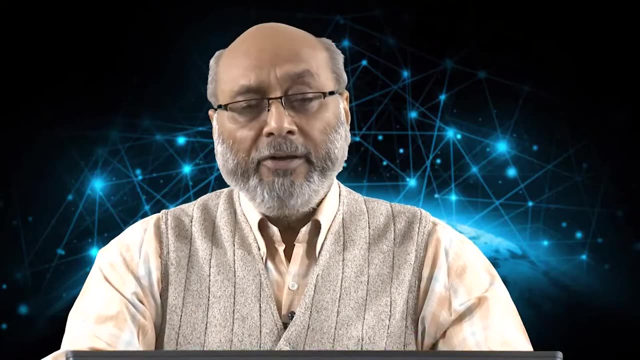 hydrologic modeling using digital elevation model to answer certain questions like: what happens when deforestation occurs? So the forest creates impediments in the flow of water over a surface. So if plantation is removed or forest is removed, what would happen to that thing? You recall the very first discussion on GIS in this course? 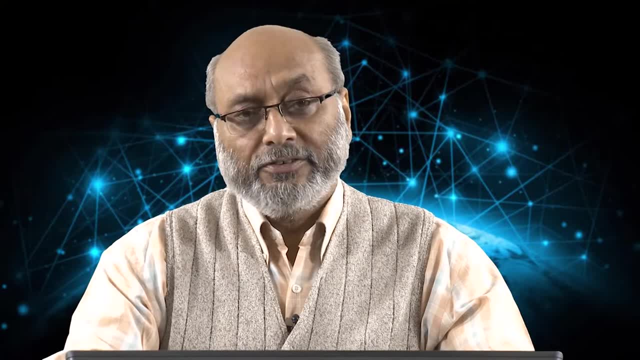 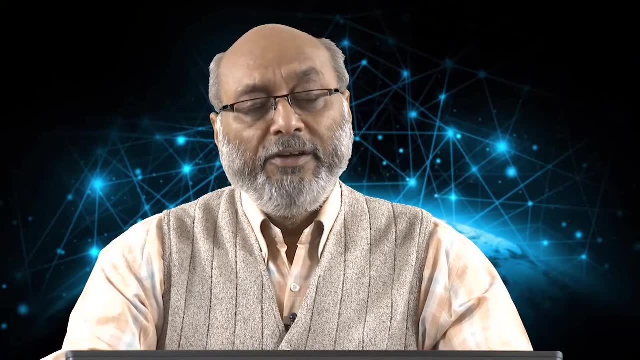 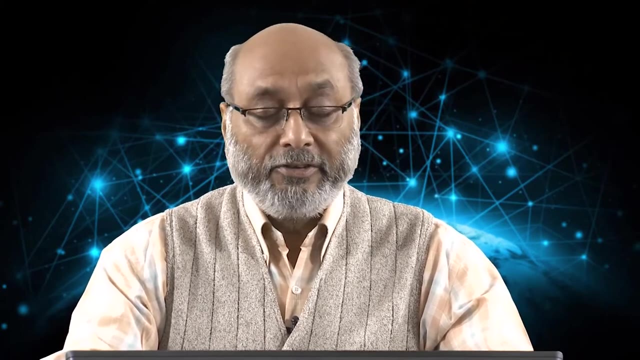 I showed one video, One watershed, through two different pictures, and there I showed that if in one area the forest is removed, deforestation takes place, then what is going to happen to the soil moisture condition in that particular watershed? And in the second scenario it was that if at 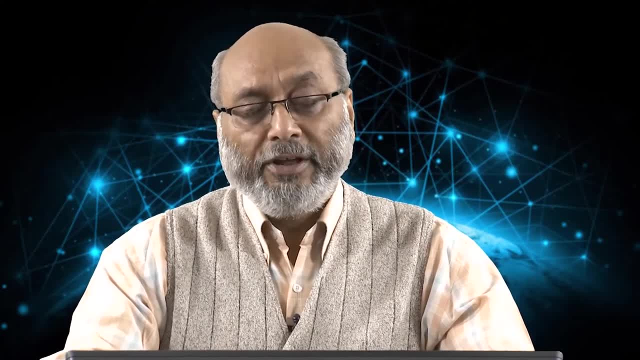 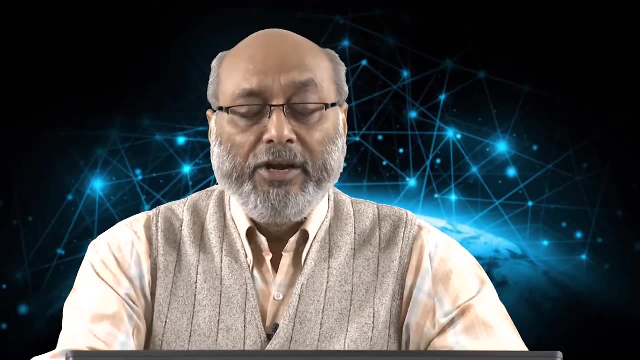 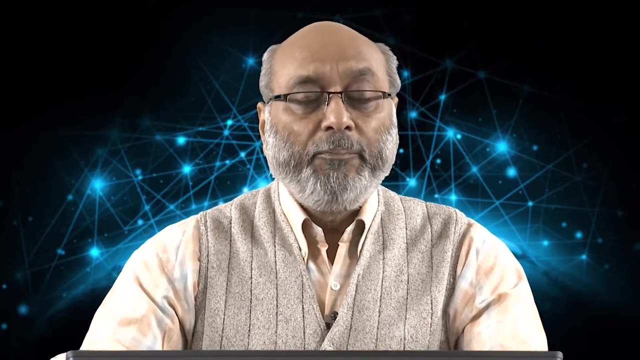 another place the same equivalent area of forest is removed, then that scenario will change. So deforestation takes place, So different conditions will bring different results, And many such things can be simulated, modelled, predicted, before anything really happens on the ground. So your GIS, your 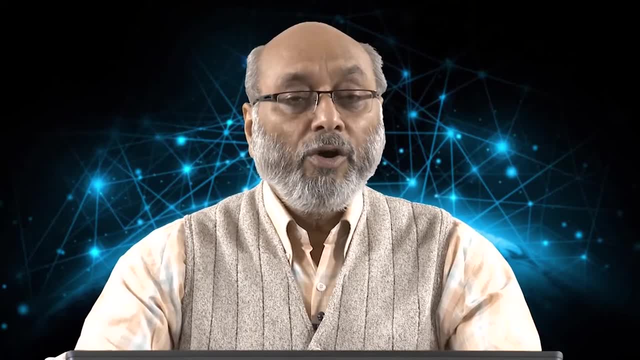 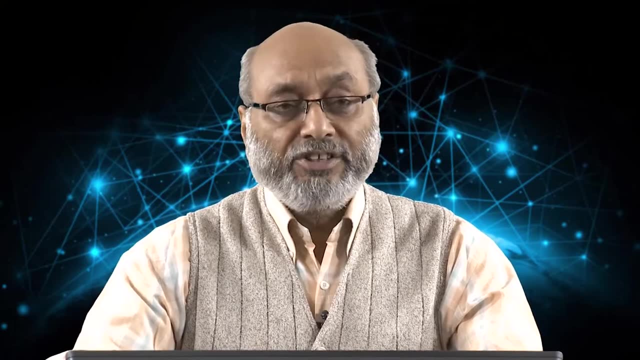 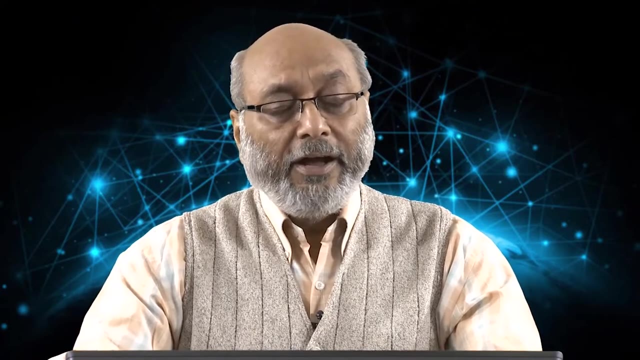 digital elevation model and surface hydrologic modeling. all will allow us to predict and see or visualize what would happen if any action is taken on the ground. Now, how does this affect the watershed? I have given the example. If deforestation occurs, it affects. 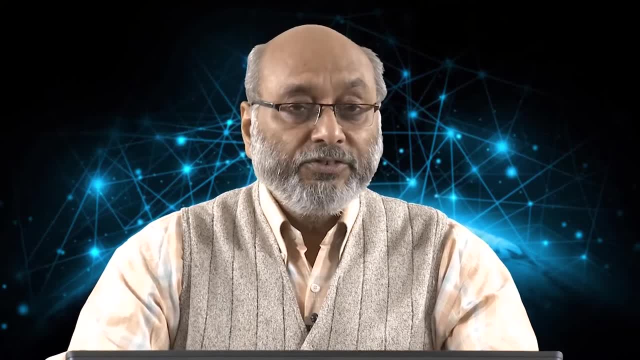 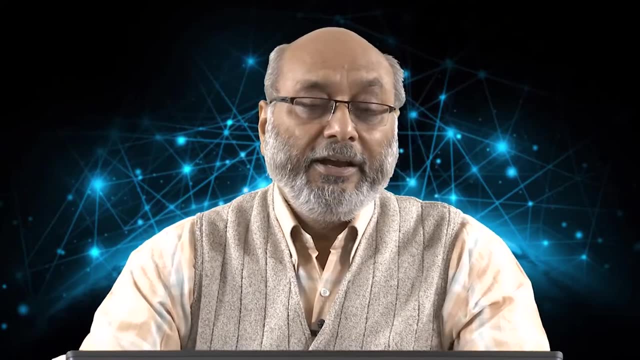 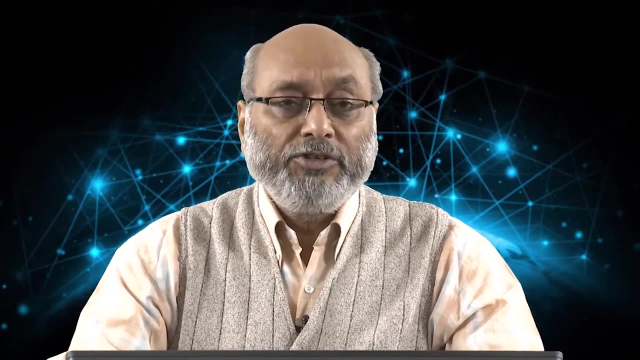 the soil moisture condition, And if soil moisture condition is changed, it will bring changes in soil erosion, It will bring changes in groundwater conditions and many other things. So any change on the ground, on the surface of the earth, which takes place in terms of 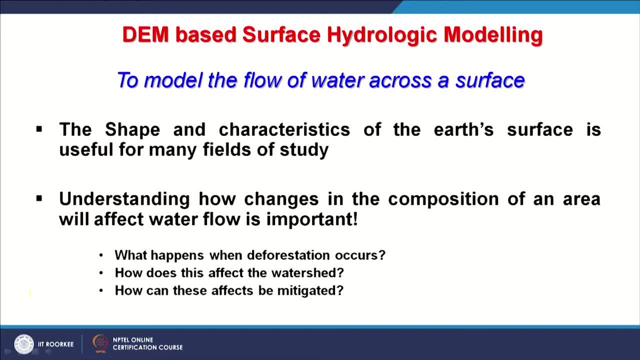 vegetation or drainage or change in elevation. All these changes will bring changes in soil elevation. All will bring changes in some way or another, Maybe immediately or maybe after sometime. It depends what action is being done on the ground. And also we can answer through this surface hydrologic modeling that how can these effects? 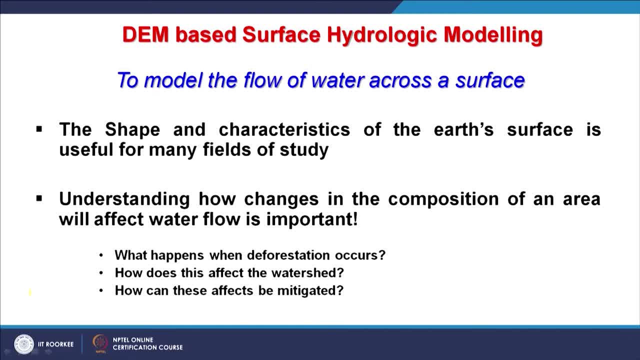 be mitigated, How we can minimize the impact, if at all the development, because development should not be stopped, It has to take place And at the same time we have to take care about the environment and surface of the land. So how best we can bring a scenario. 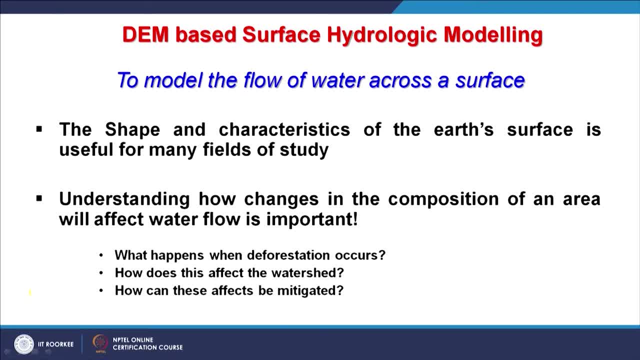 where minimum damage occurs to the environment, So that can also be modeled through GIS and surface hydrologic model, And therefore this combination of digital elevation model and surface hydrologic modeling in GIS has brought many applications which we will see, even how these will be implemented. 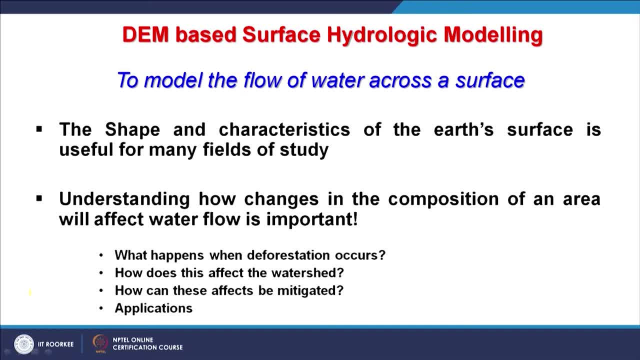 These will affect the groundwater conditions or how we can think or visualize the groundwater conditions or changes in groundwater conditions can also be there. So not only in civil engineering, in hydrology, in earth sciences, but in various domains these applications are there. 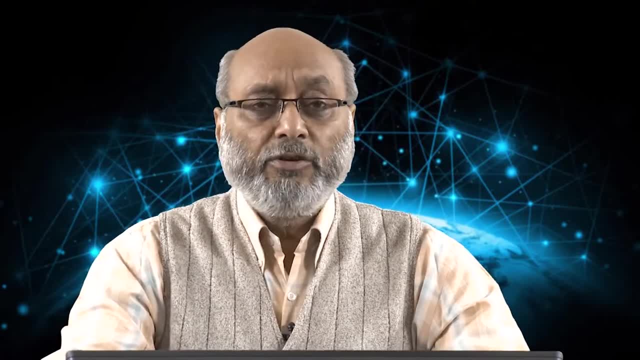 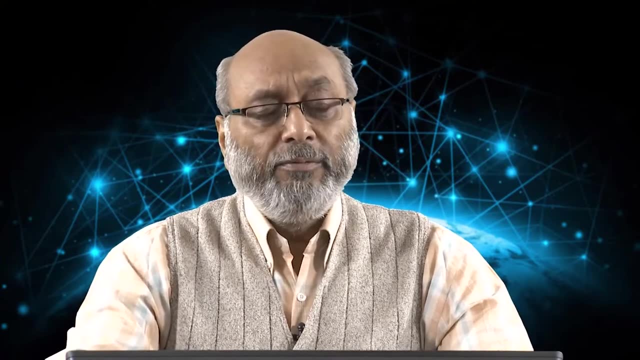 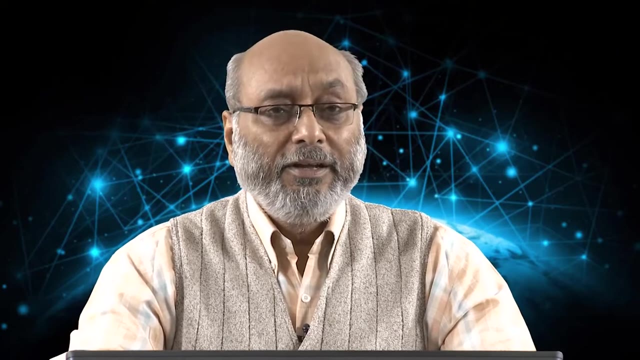 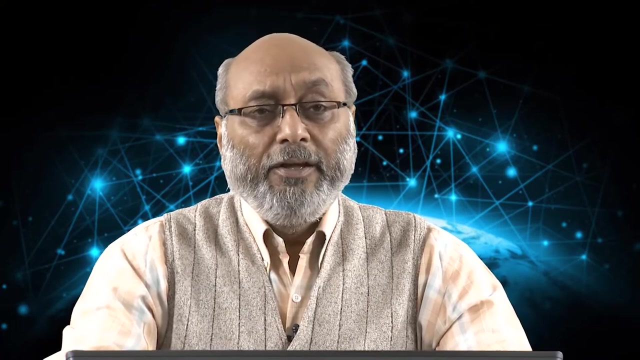 Now, before we really go for this surface hydrologic modeling, we have to understand how water flows on the surface and how it develops a drainage system, Because this surface runoff is not uniform throughout the surface of the earth. So it basically develops the drainage system, or river network, or stream network, So basically, 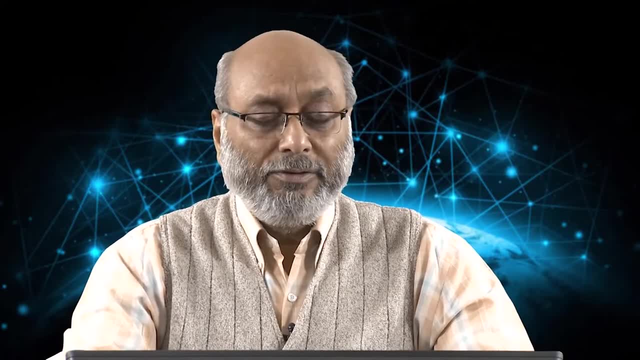 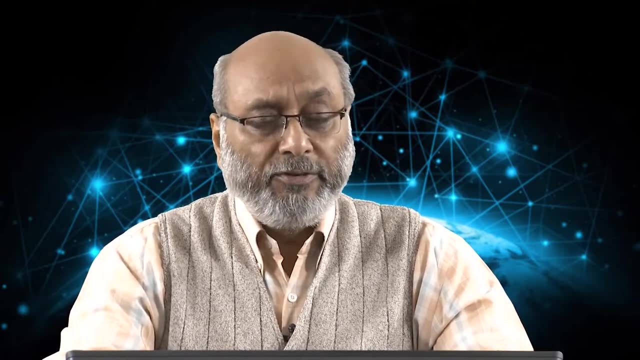 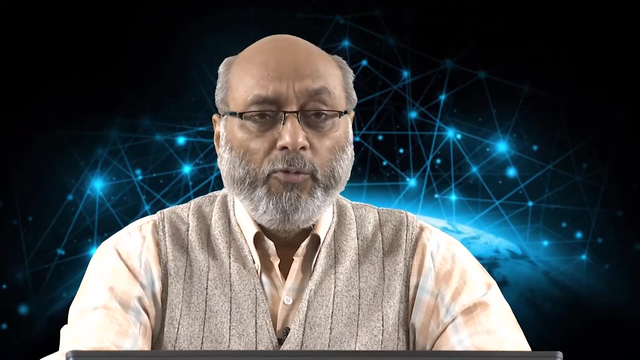 what it means that the area upon which water falls. basically this includes all kind of forms of water. So in total, we say precipitation and when we say rainfall it means only water in form of liquid. So whatever the precipitation which occurs on the surface of the earth, ultimately it 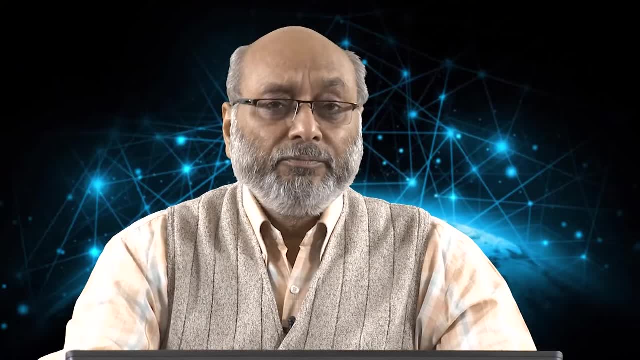 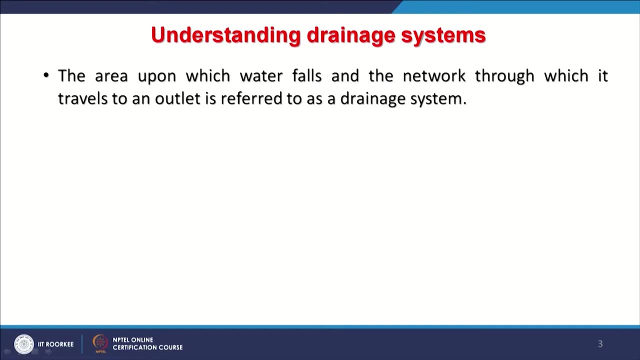 will go through or move through the network which is our drainage network and through which it travels to an outlet that is a watershed outlet or basin outlet, And entire this thing where it happens is called the drainage system. So flow of water through a drainage system. 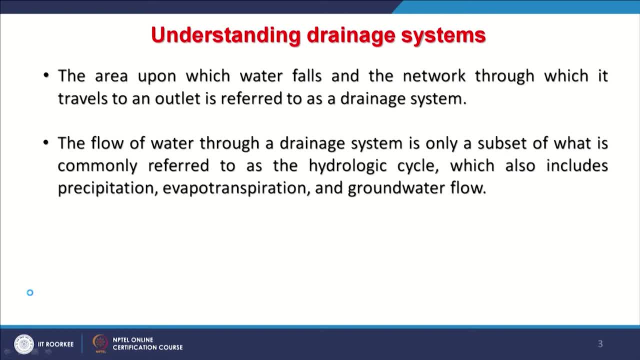 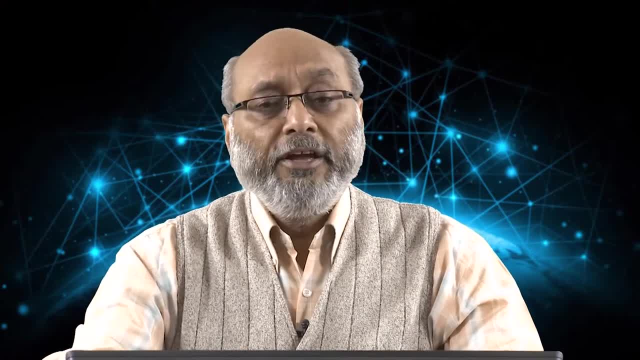 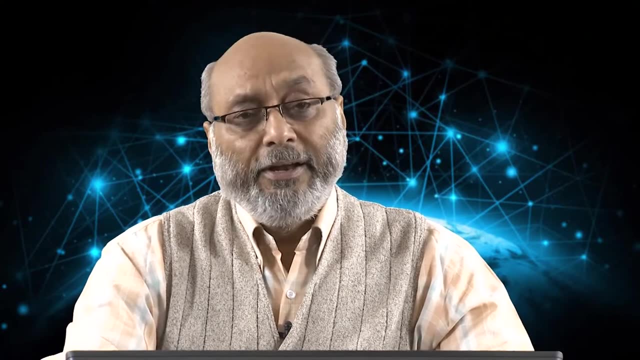 is only a subset of what is commonly referred as part of hydrologic cycle, Because hydrologic cycle is big, even the water which is going through evapotranspiration and then it goes in the atmosphere, it condenses, rain occurs or precipitation occurs, and then 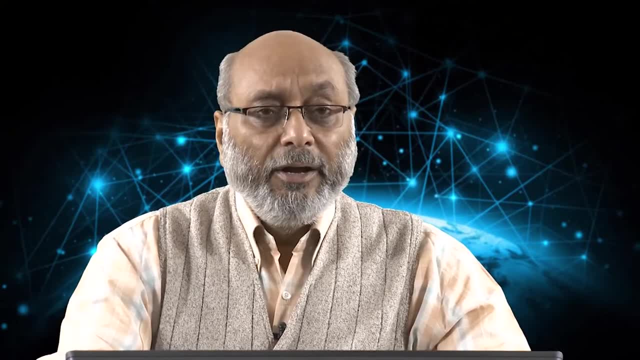 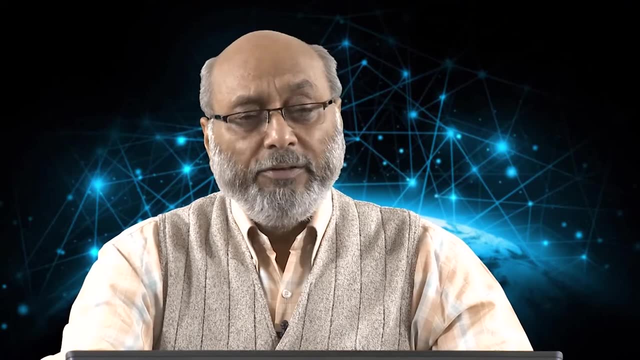 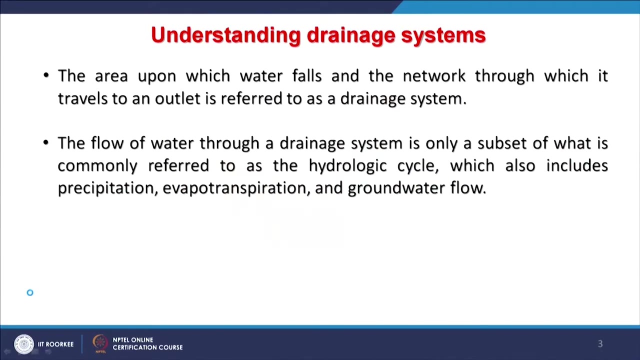 again it flows. So hydrologic cycle is very big, But there is a contribution of drainage to hydrologic cycle And whatever is the part of hydrologic cycle which also includes, as I have mentioned, precipitation, evapotranspiration and also groundwater flow. 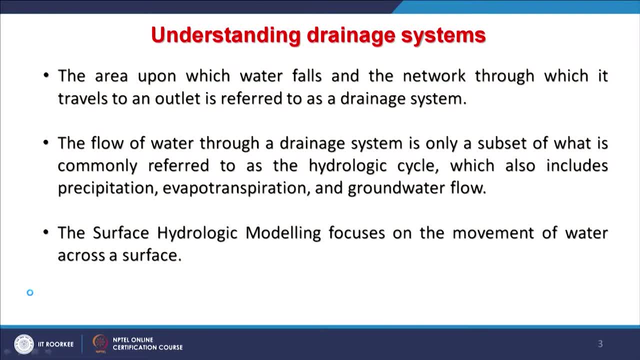 Surface hydrologic modelling basically focuses on the movement of water across a surface or over the land, How water will flow, How this surface runoff will occur. Now, further, in order to develop the hydrologic model, we have to develop the hydrologic model. So 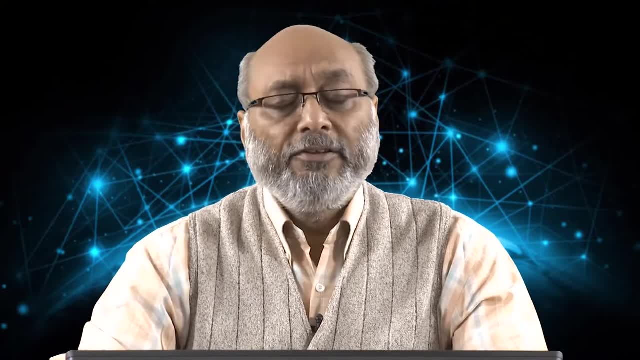 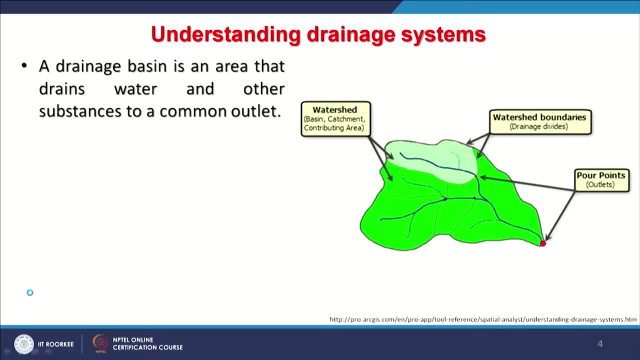 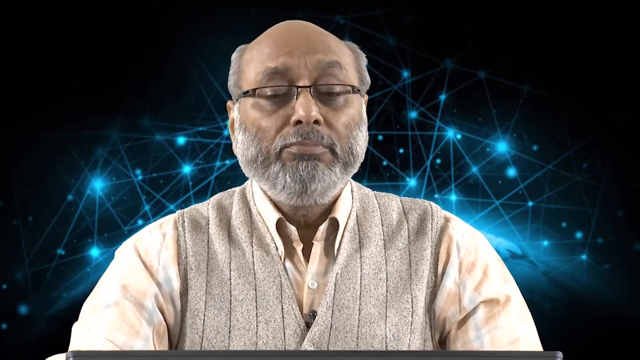 to develop our basic understanding before we go for real surface hydrologic modelling. we have to also understand. a drainage basin or drainage system is an area that drains water and other substances to a common outlet. Now, other substances might be your sediments, very common. other substance may be pollutants or may be other like wood and other materials. 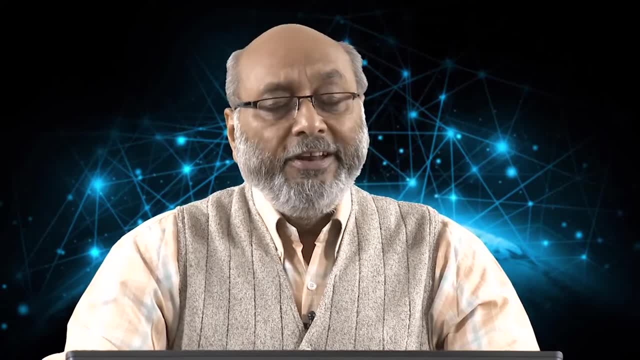 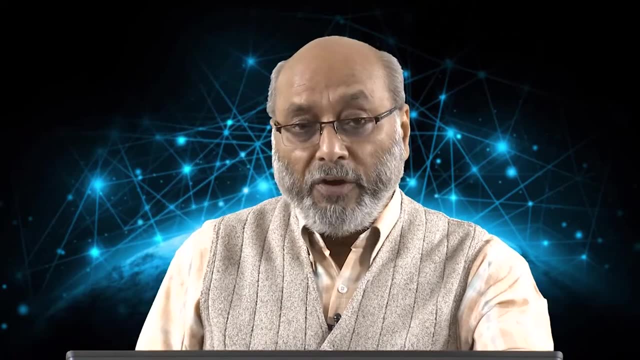 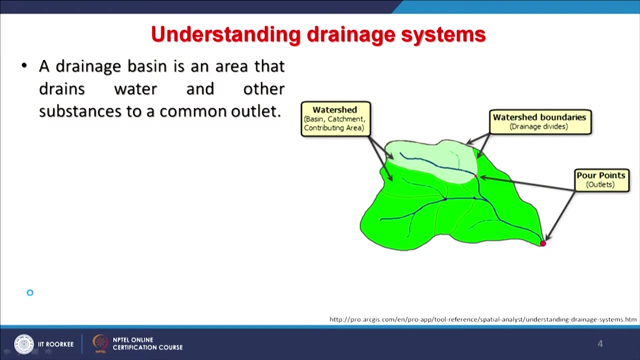 So all these are carried Through this drainage system by the water. Here some terminology which we will be using. So those who are not familiar about this, for them it is fresh. but those who are know, it is refreshing for them that the important point here is this outlet of the watershed. 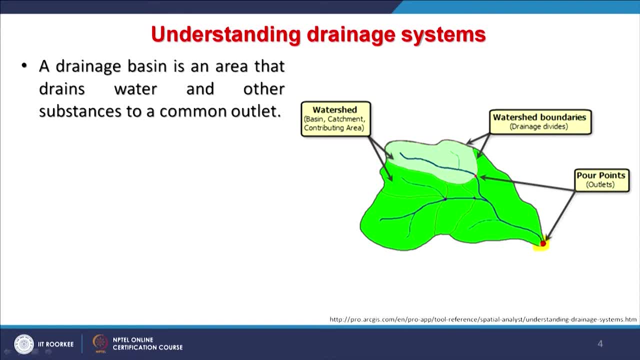 And this topographic high which is creating a watershed or boundary, topographic boundary, is called basically watershed or drainage divides. It also called drainage divide. Why drainage divide? Because whatever the drainage network which we are seeing is all contributing to this outlet And the interesting part is that one watershed- 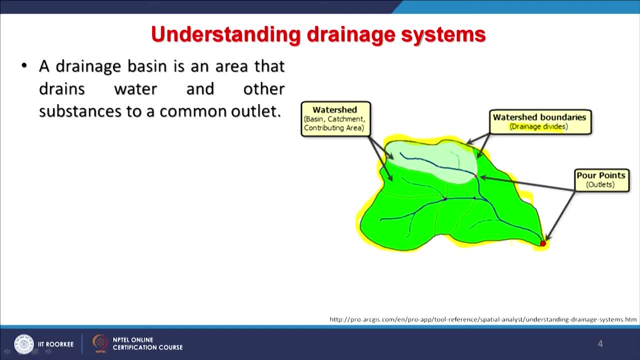 ends, another watershed starts over the land. So over the entire globe, there is a continuous. This is continuous. The size and shape of watershed may change. That adjacent watershed may have a completely different shape and size, But one watershed ends, another starts. 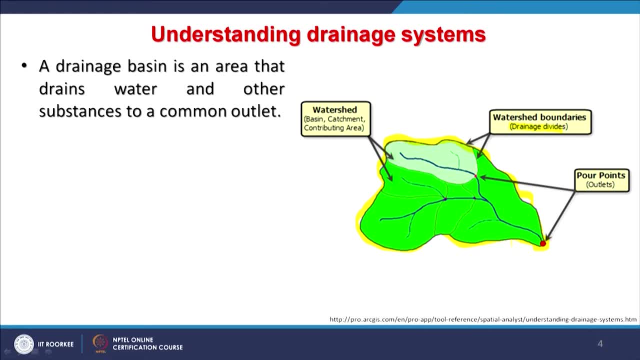 And all over the land of the earth. this is true Now, watershed, but same time we also use some other words like basin and catchment. All are contributory areas, Basically what they are doing, Whatever the precipitation occurs in this drainage divide or topographic. 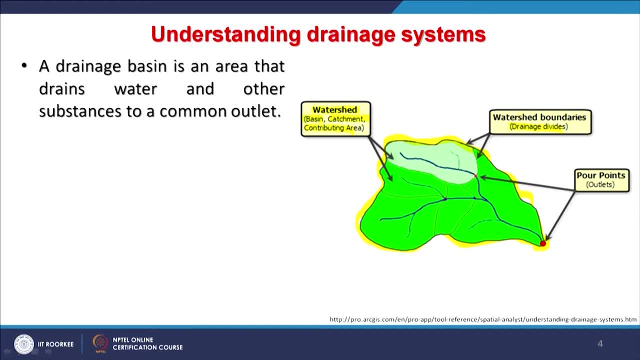 high area which is depicted through this watershed boundaries. whatever the precipitation will occur within this boundary has to come out from this pore point or outlet. There may be some loss of water Into the atmosphere through the processes of evapotranspiration, or there may be some loss of water into subsurface through groundwater. 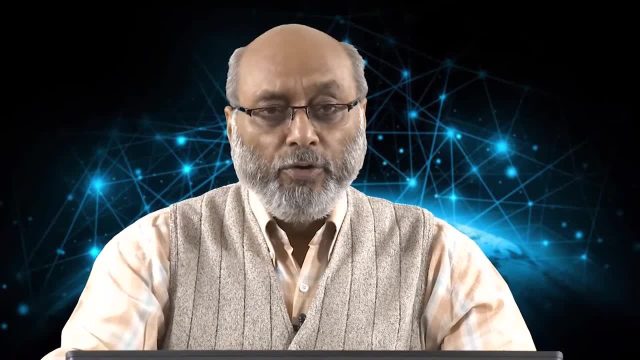 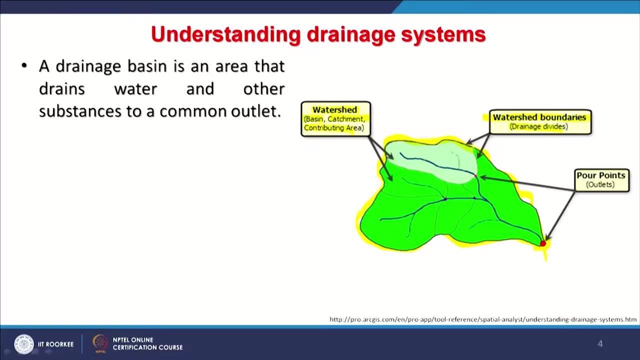 So if we exclude, then whatever is surface runoff which will occur, which has to come out from this outlet Now, within a watershed we can also have subwatersheds, like here. it is shown in a light green colour. So even a large surface runoff can occur, even a little water loss can occur. So 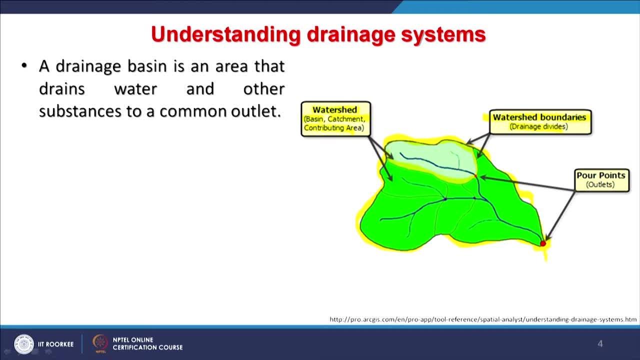 So each drainage line or stream can have its own watershed. For example, I do not have currently the topographic map of this digital elevation model in the background, But if I decide that this is my outlet, then this can be my watershed, like this: 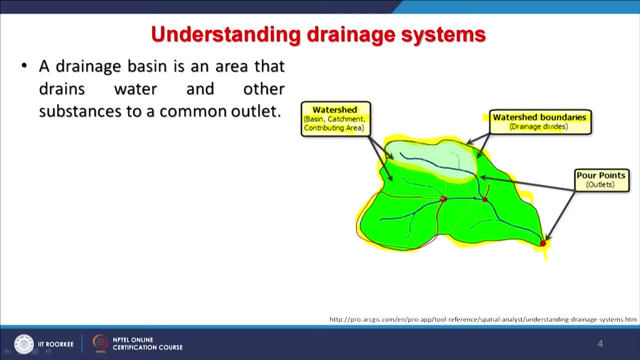 And if I decide that this is the outlet, then this can be my watershed. So as you go lower and lower towards the outlet, the watershed or sub-watershed becomes larger and larger, And as I go higher and higher in the order of stream. so this we say: first order stream. 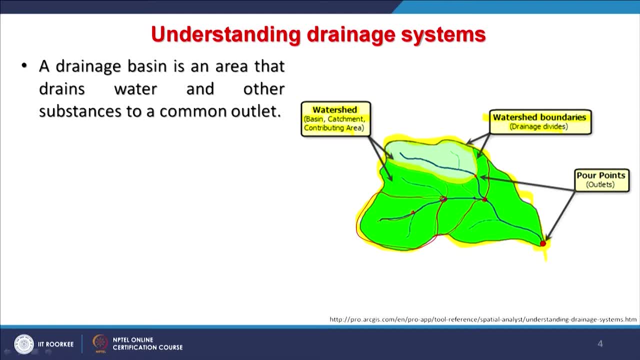 We will have full discussion on this. So if I decide, my outlet is here. this watershed is going to be only this much. So within a watershed we can have many sub-watersheds. Now other common terms for drainage area. I have just mentioned that watershed basin. 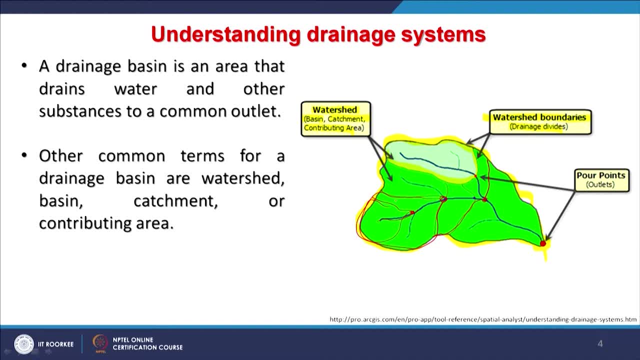 catchment or contributory area. Whenever we use word watershed or catchment, catchment is used in other domain also and can bring some confusion also, But when we say watershed it is really related with high-level drainage. So it is related with high-level drainage. 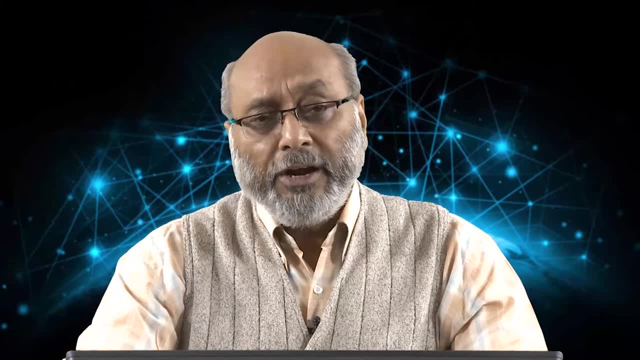 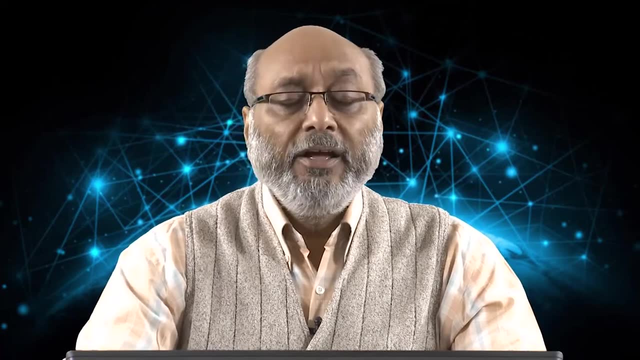 And whenever we say watershed, it means we are not talking of a very large area, And when we say basin, we are talking about a very large area. For example, we will say Ganga basin, we will not say Ganga watershed or Ganga catchment. 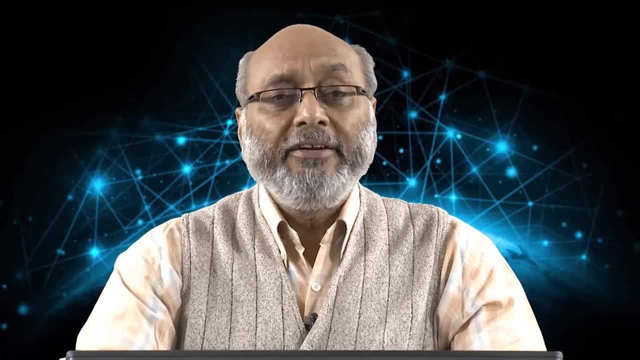 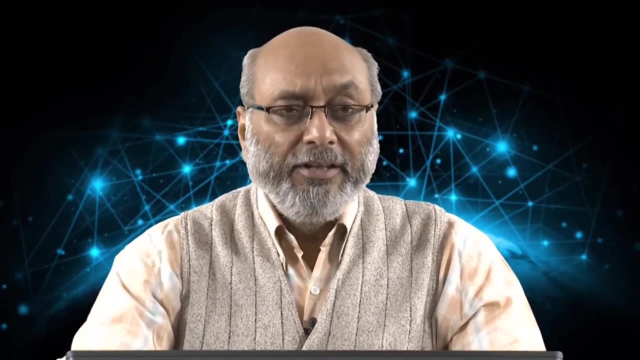 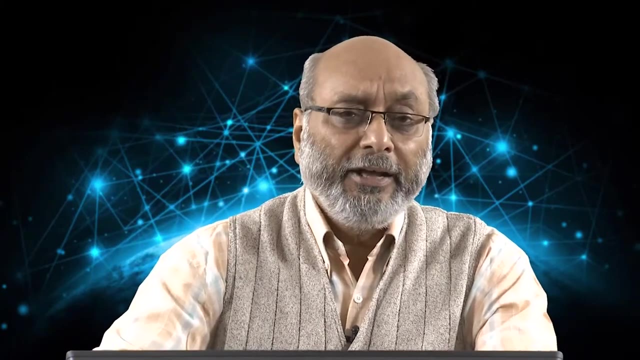 So there is some difference, but there is no quantity attached to this, that if a watershed is more than 100 square kilometer it would be called basin. There is no such classification. So generally for a smaller basin, For a relatively smaller size, we use word either watershed or catchment, and when it. 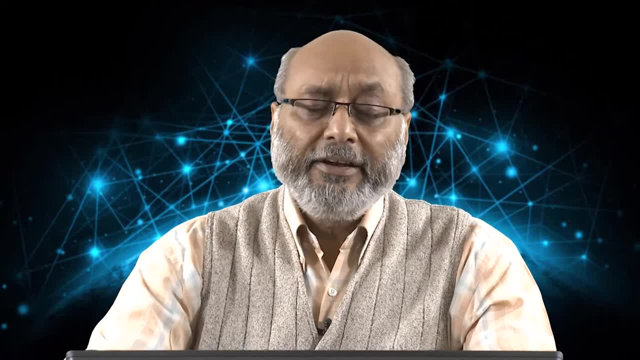 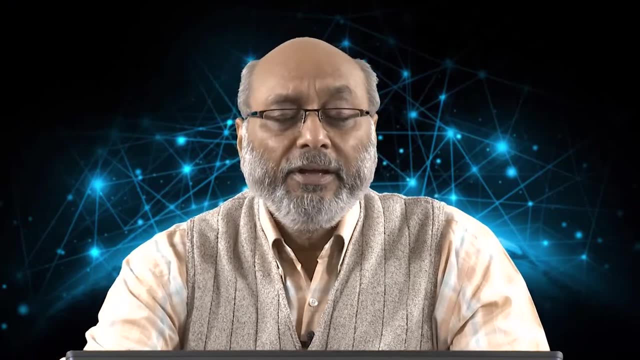 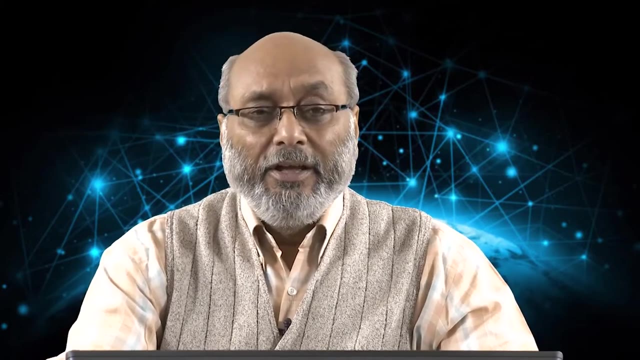 is very large area and this watershed, then it becomes basin or contributory area also And in a canal system we will call them as a distributory area or command area, which is just opposite to the watershed or basin. So this area, that is, the watershed area, it is commonly or normally defined as the 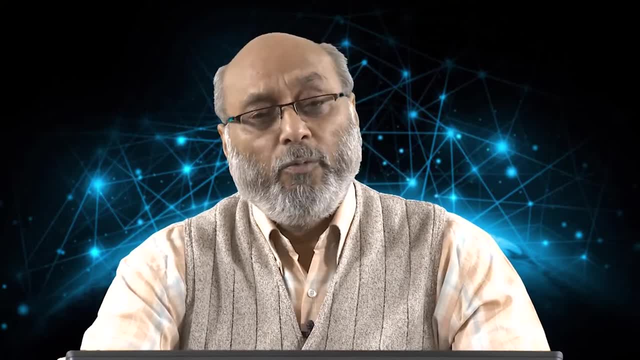 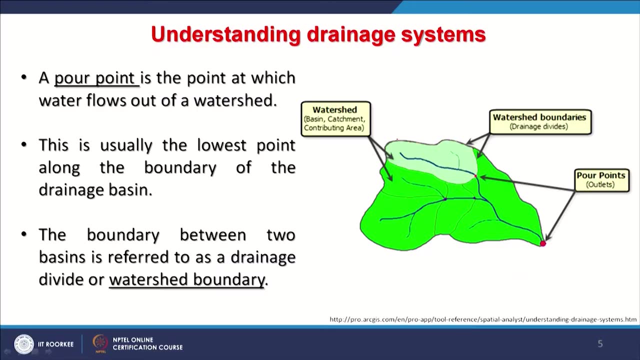 total area flowing to a given outlet or pour point. Now, pour point I have just explained. that is the point at which water flows out of the watershed. So it may go out of one watershed but may enter in the larger watershed or a larger. 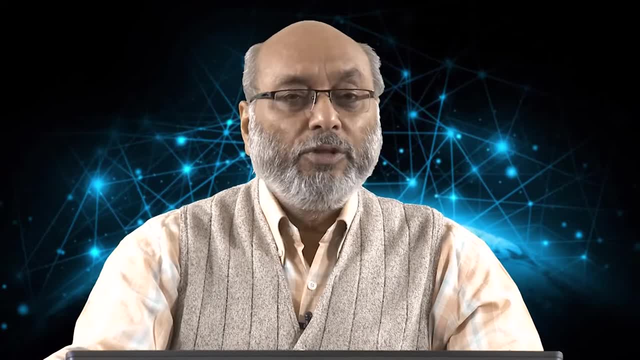 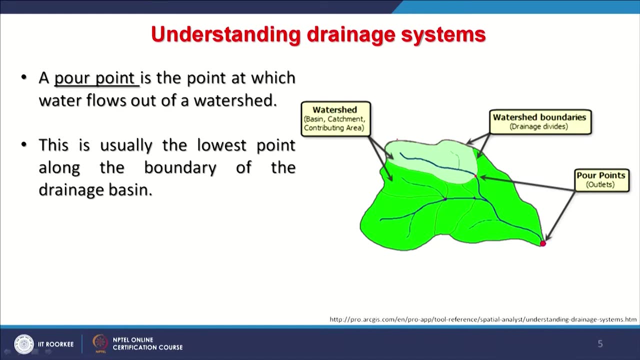 basin till it reaches to the sea, And this water outlet is generally, or usually, the lowest point along the boundary of the drainage basin. It has to be the lowest, So whatever the precipitation is occurring will come out through this outlet, And the boundary between two basins or watershed is defined as a drainage divide or watershed. 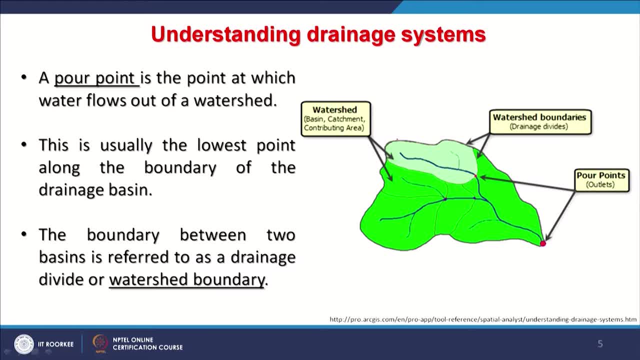 boundary. So if this is the boundary and if rainfall occurs here and surface runoff occurs, it will come out from here. But if rainfall occurs there, Then there will be another watershed and the outlet might be in this direction. So that will come out like this. 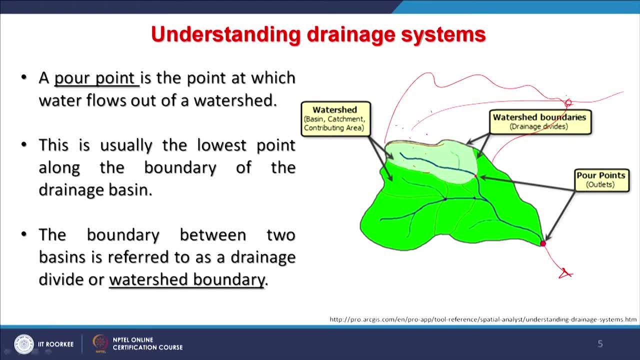 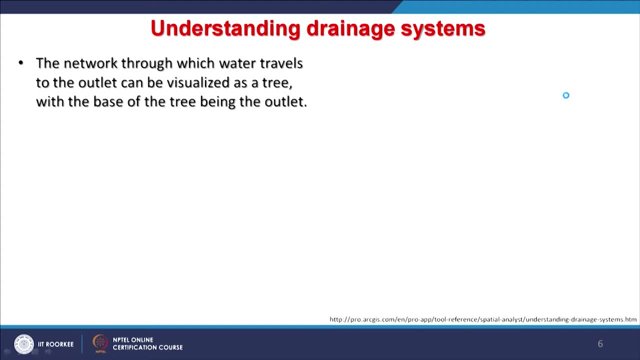 So this becomes the outlet for that. So basically, it is also the precipitation which falls in. whatever in the boundary will come out through surface runoff. Now these drainage network or stream network which we see in form of these- generally they are represented in maps- 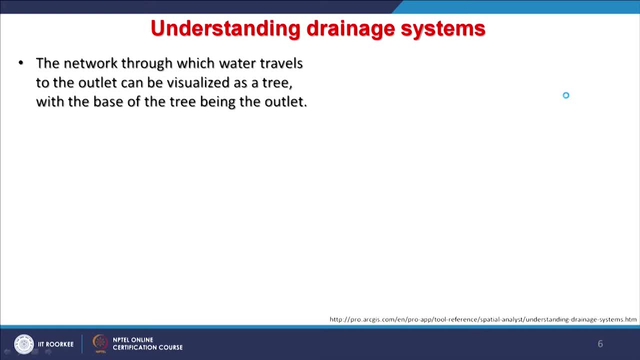 In blue lines or black lines. this drainage network through which water travels to the outlet can be visualized as a tree with the base of the tree is at the outlet, as you have also seen here, Like here. what do you see? that this is my base of tree and these are the branches which 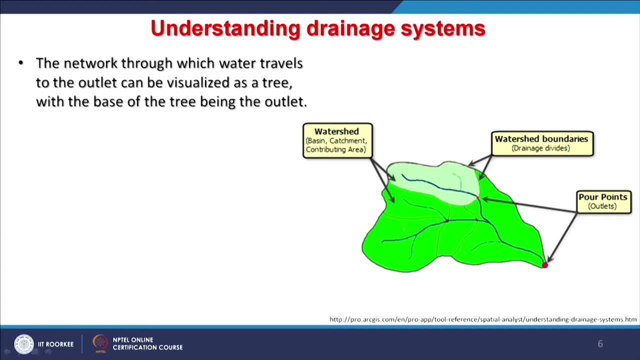 are other lower order streams. Now the branches of the tree are the stream, These are the stream channels, And the intersection of two stream channels is referred as a node, or jang sang So in GIS. So here this may be one stream, same first order stream and this is also first order. 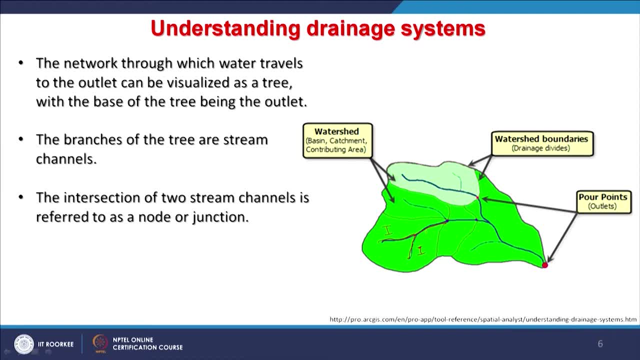 Now, when two first order streams meets in one scheme, they become second order, And likewise we keep adding. So that means the intersection of two streams. So two stream channels is referred as a node or a jang sang, or for downstream it may become 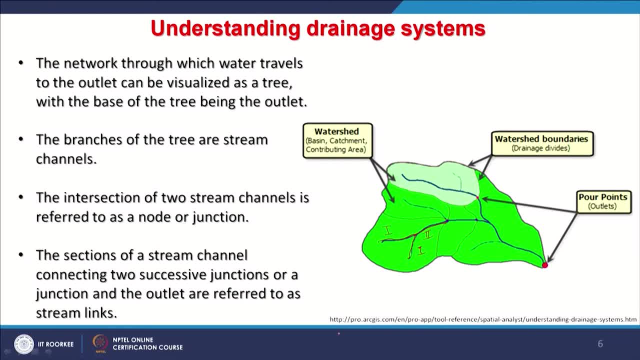 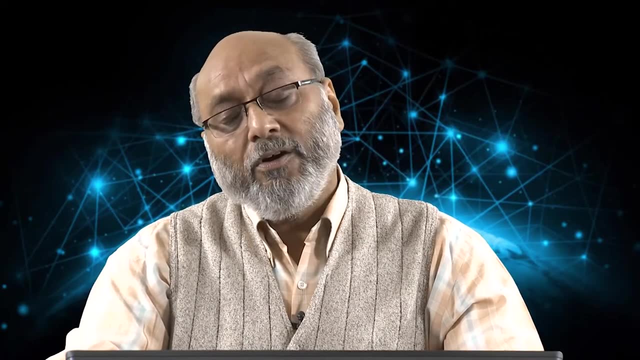 another order And sections of a stream channel connecting two successive jang sang or jang sang. at end the outlet are referred as the stream links. These stream links are very important while deciding the order of the streams. So through surface hydrologic modelling, 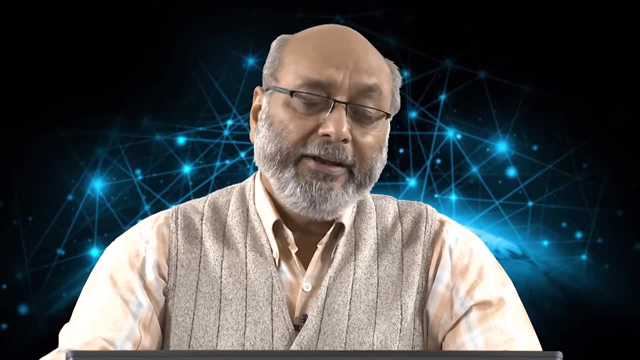 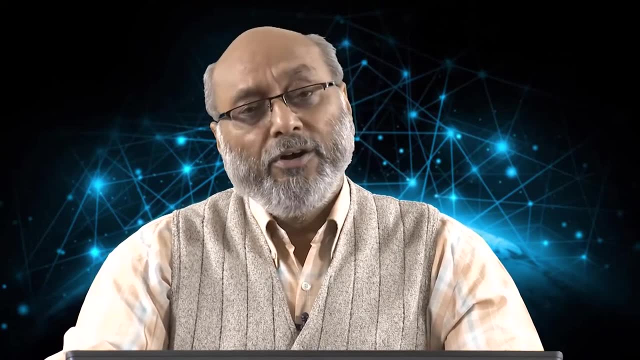 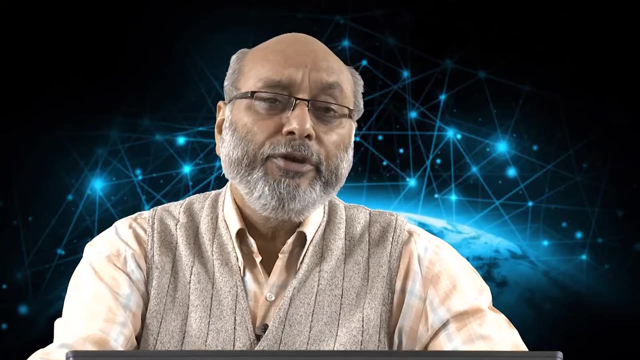 Yeah, derivative can also come that, whether streams are following, there are 2 well-known, well-established methods, whether stream method or stream method, which we will discuss later Now. as I have been saying, it is a topographic divide. Watershed boundary is also a topographic. 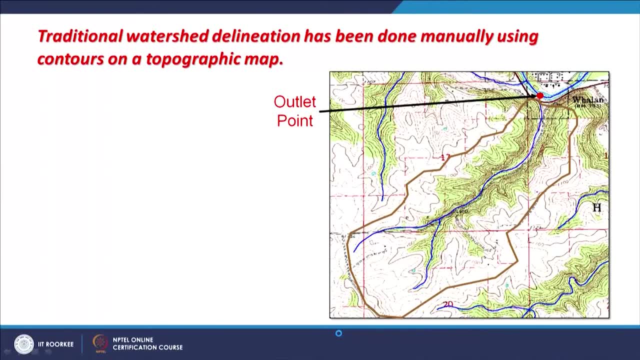 divide. So if you see a map which is a topographic map and wherever you are having higher points or contours are having like this, or spot heights are also there, then that becomes the watershed boundary. So using a toposheet and with some care, we can definitely draw a watershed boundary. 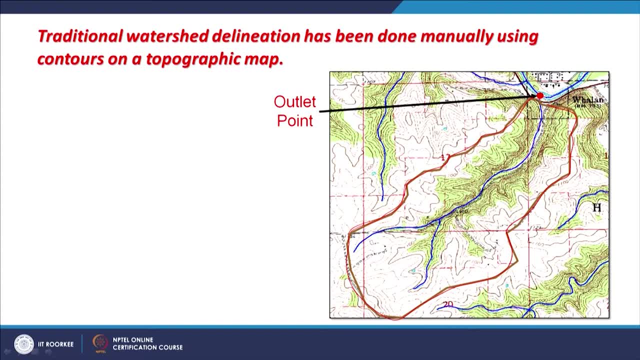 quite easily. But if we are having GIS and digital elevation model, we can do all these things very accurately and automatically through this surface hard logic model. So traditional watershed delineation, which we have been doing earlier when we did not have the GIS and digital elevation model. 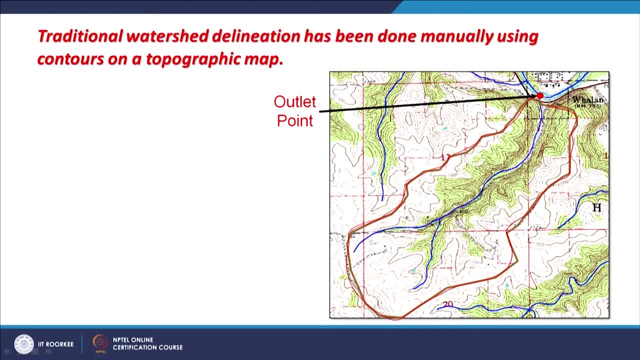 like today, by using contours on a topographic map And a watershed. boundary can also be, as how you start doing or drawing on a toposheet, that first you decide which is going to be your outlet, like in this case, And then you start searching a boundary, or that is through GIS. 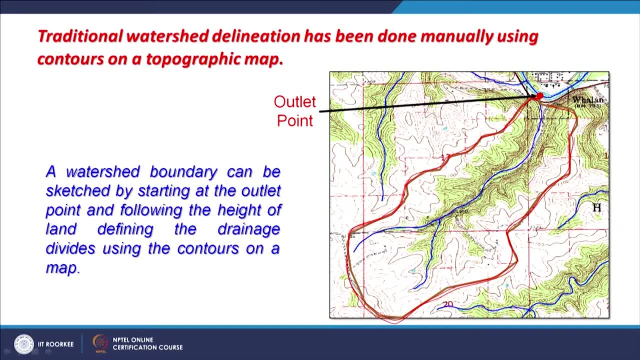 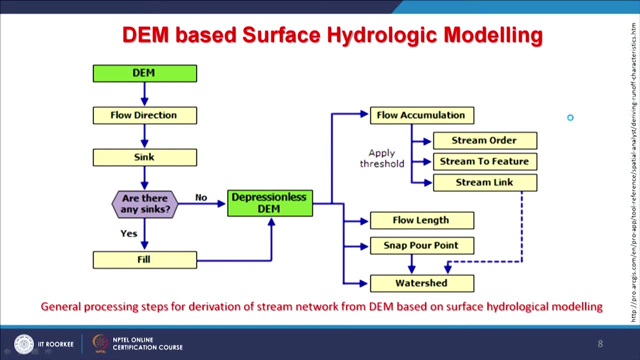 Through your contour lines or a ridge and by which then you complete the entire watershed boundary and you come back to the same outlet. Now let us discuss a surface hard logic model. So far, we have developed some basic background about some you know terms which we will be. 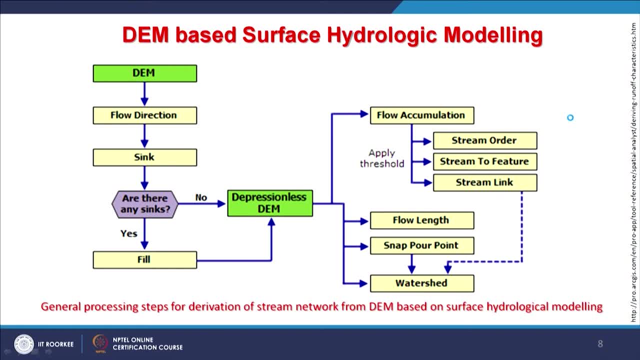 using here Now this first and the only input basically is required initially. This is the digital elevation model. Interesting thing here is that surface hard logic modelling is more or less sequential, So in that way it is very simple to understand. And second, 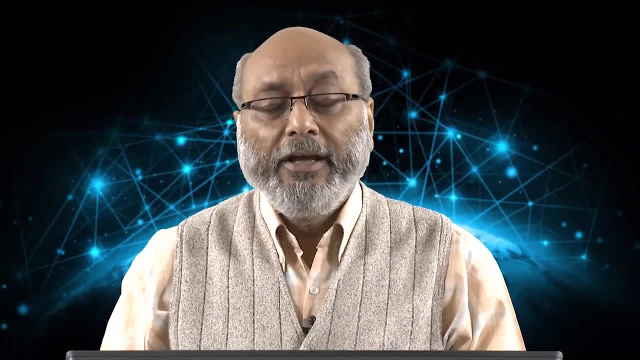 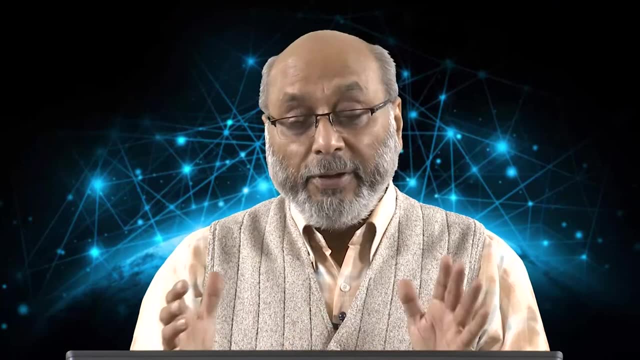 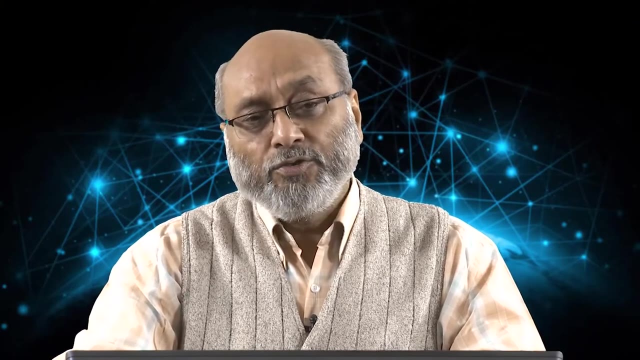 and most important thing in surface hard logic modelling is that we are having one assumption, a belief Assumption is here, which is a very big assumption. The assumption is that, whatever the precipitation will occur, It has to come out through the outlet, and that means we are assuming that there is no. 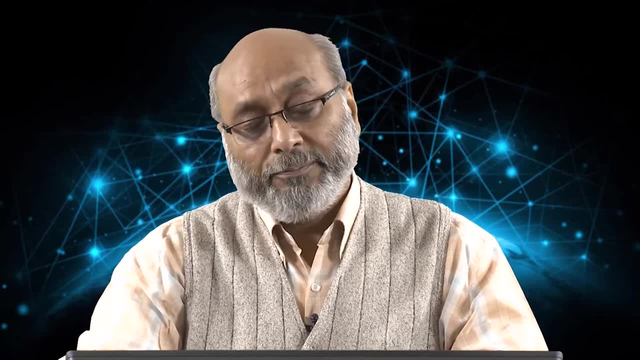 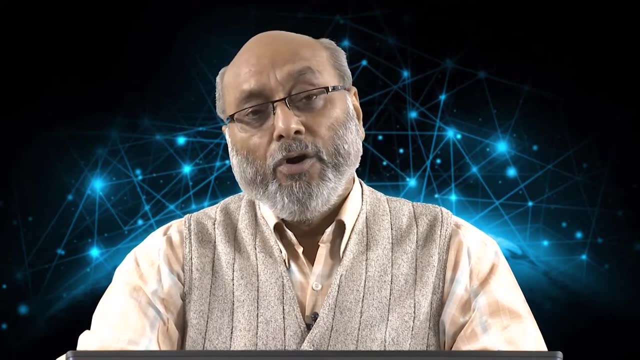 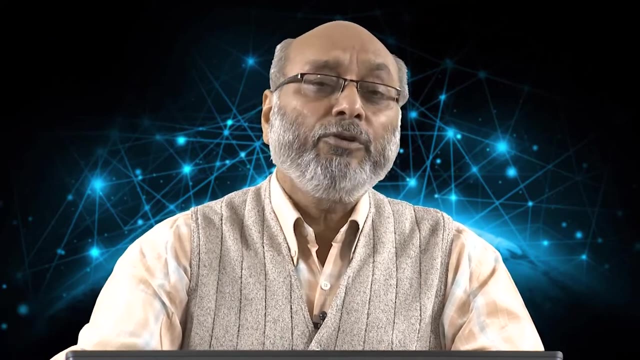 loss of precipitation or no loss of rainwater, neither to the atmosphere, through this evapotransmission, or neither to the ground nor to the groundwater. So, whatever the water, even a single drop, if it falls in a watershed it has to come out of it. 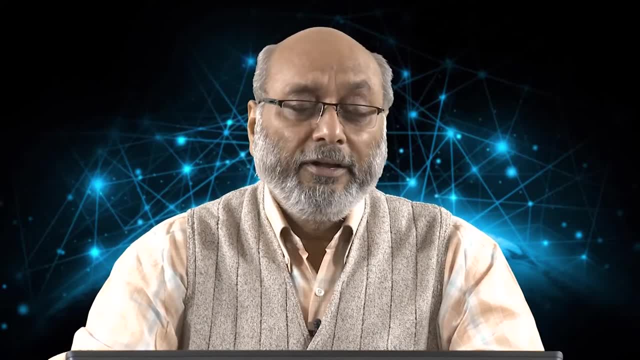 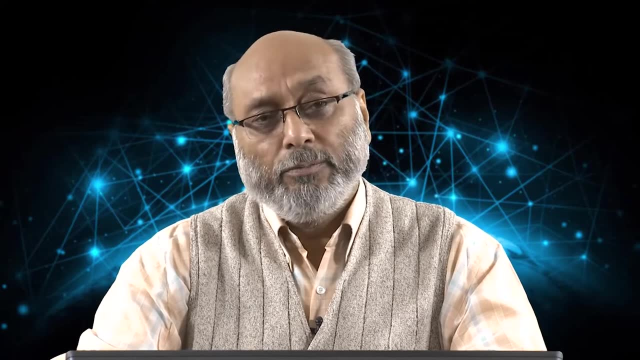 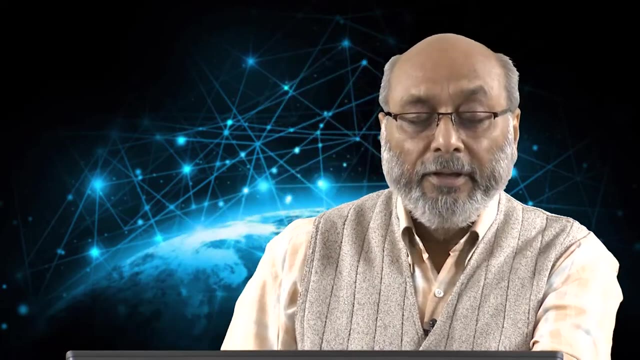 It has to come out of your outlet or out of your watershed. This is the only assumption in surface hard logic modelling. So input is digital elevation model. The first thing which we do generally is we drive the flow direction. Flow direction is more or less. 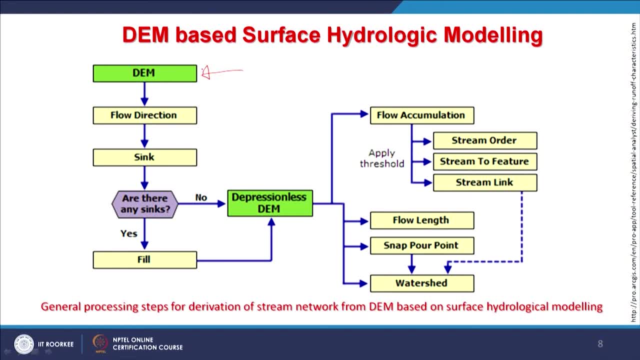 like your- you know- slope map. Then we identify the sinks. Why sinks? Because this is what I just mentioned about assumption: The sinks are the depression artifacts, error within your digital elevation model. So, again, a 3x3 kernel will be used and if any cell is found that there is water will. 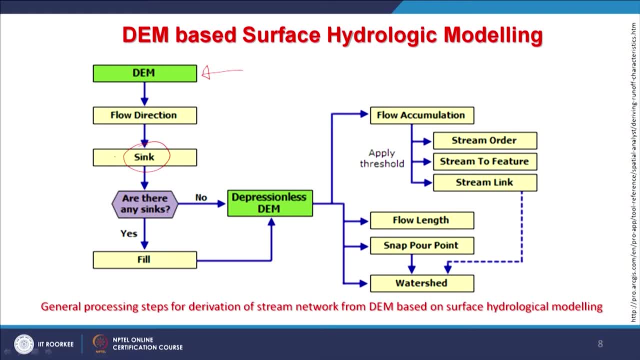 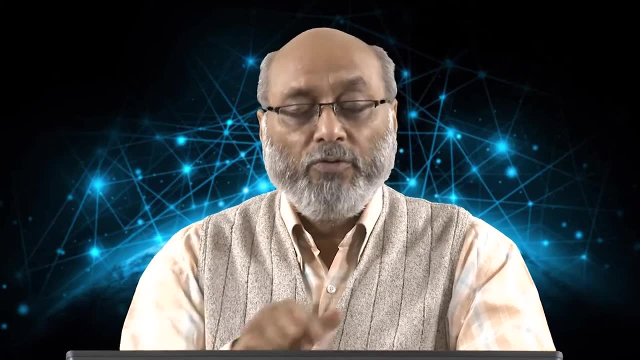 not flow out of that cell, then it is labelled using the surrounding 8-pick 8 cells values. it is labeled That means the sink is filled and that means the water then will flow. Otherwise there will be stagnation of water in that lowest cell out of 8 surrounding cells. 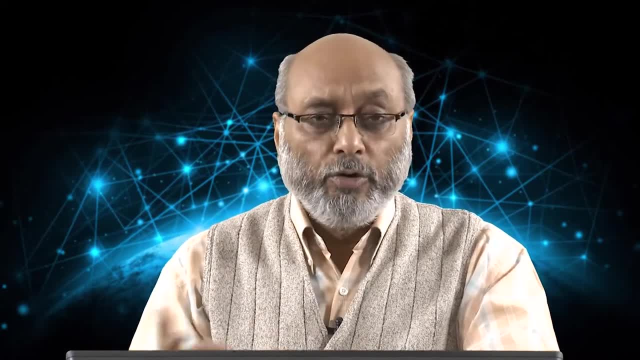 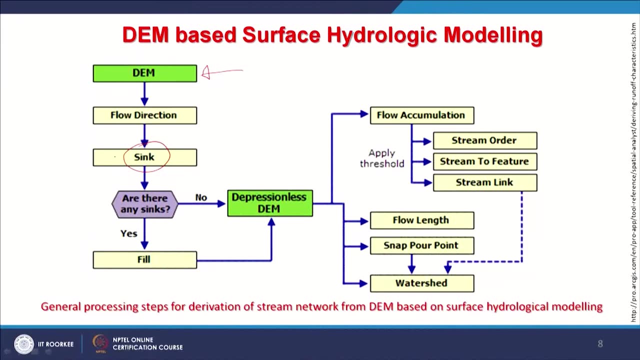 So sink identification has to be done. I will show you some images also, or a DM with sinks, And then, once you have identified the sink, you are already having one output, which is flow direction. Now you have to fill these sinks. no problem, There are algorithms. the 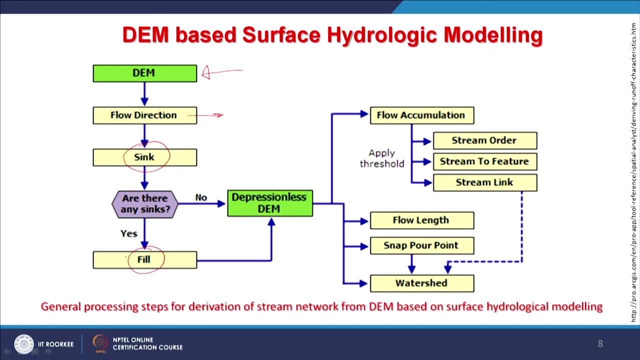 software is there and very easily you can fill the sinks. So now you are having a digital elevation model which is devoid of sinks or depressions which you have already identified and filled them. Now your digital elevation model, after the sink fill, becomes a depression-less. 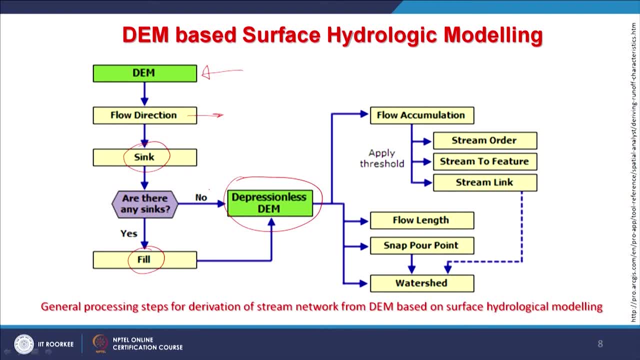 DM or sink proof digital elevation model. Now this will go for further processing and the next step, to calculate flow accumulation. Once flow accumulation has been calculated, what exactly flow accumulation is, What is flow direction? We will be discussing subsequently within this lecture or in next one. 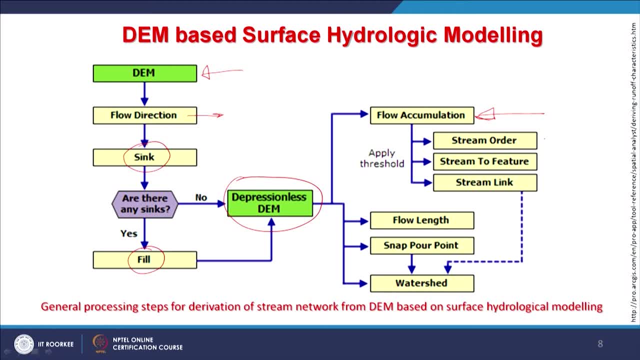 Now, using this flow accumulation, we can calculate flow direction. Now, using this flow accumulation, one can drive stream order using two Bell Stabilization methods. You can drive stream to feature, that means the drainage network, in vector form, in polyline form And also you can 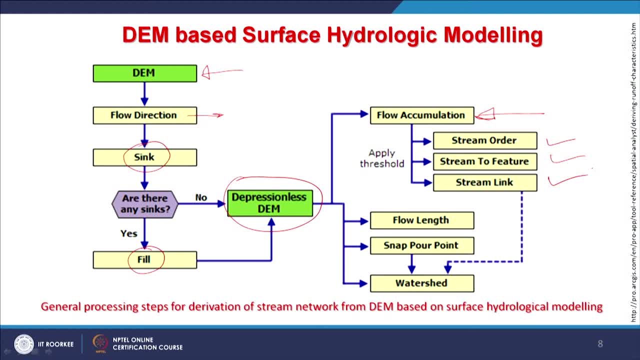 drive stream link, which are again very useful for flow modelling point of view. Further, using this depression-less digital elevation model, you can calculate flow to length. You can also get a snap pour point. that means manually: wherever you will click a watershed boundary can be delineated. And then, finally, for your input, digital elevation. 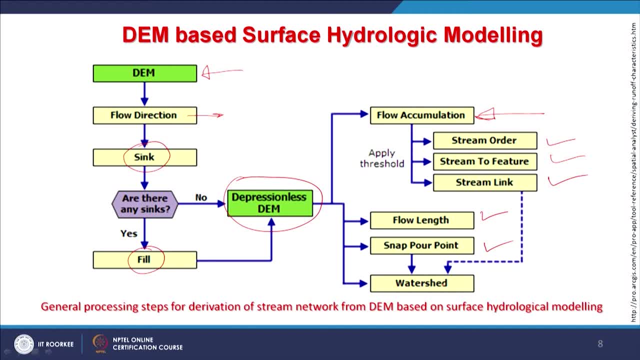 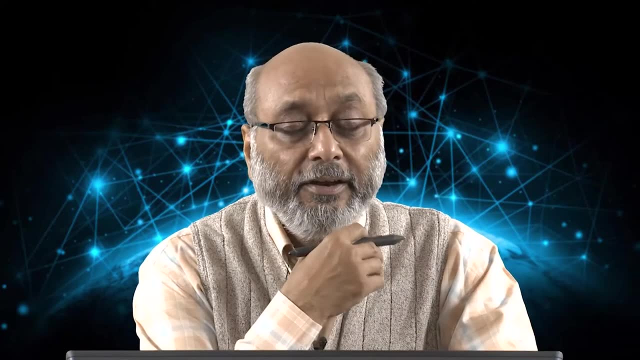 model. just giving the threshold value, you can delineate watershed, whichever the present in your digital elevation model. The only problem which you will face in the boundary areas Because, as I have said in the early discussion, that one watershed ends, another starts. So 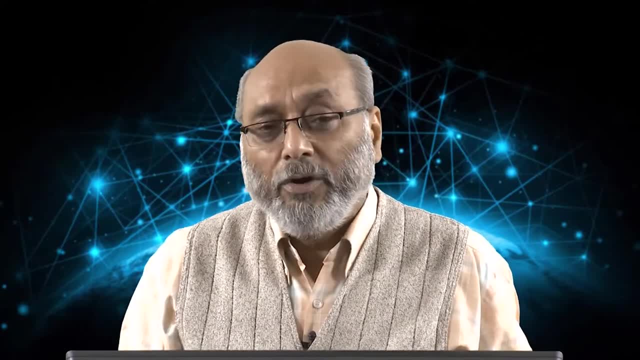 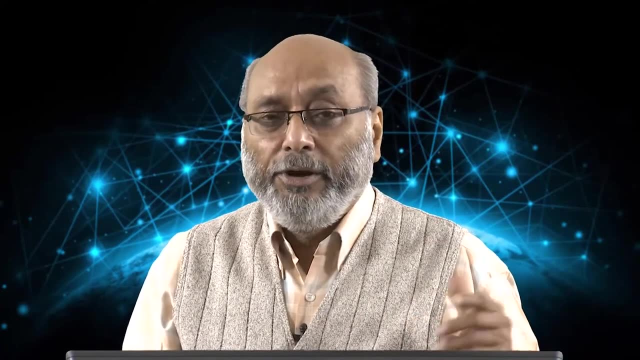 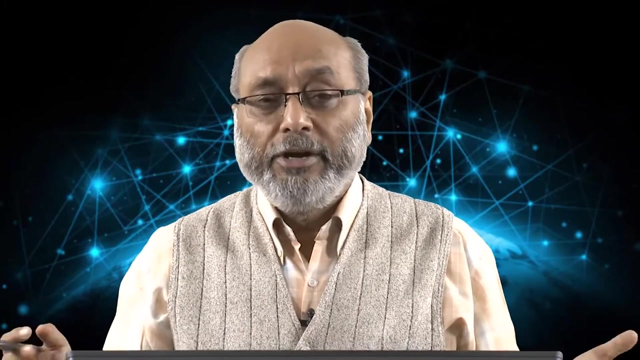 when you are having a boundary or margin of a digital elevation model. there you do not get the watershed in the adjacent, So only that part will have a limitation- not really error, but limitation. Otherwise, within that digital elevation model you can drive watersheds. 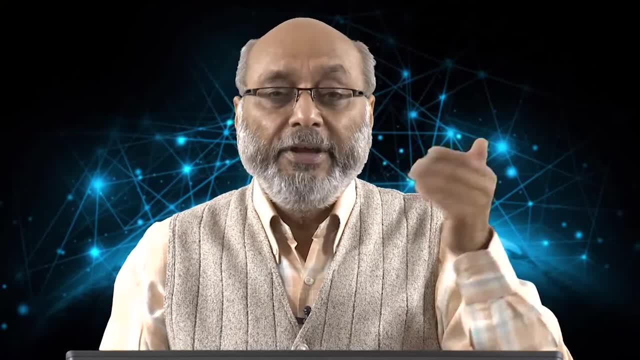 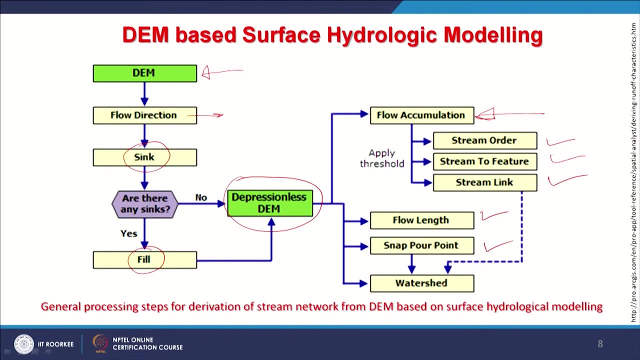 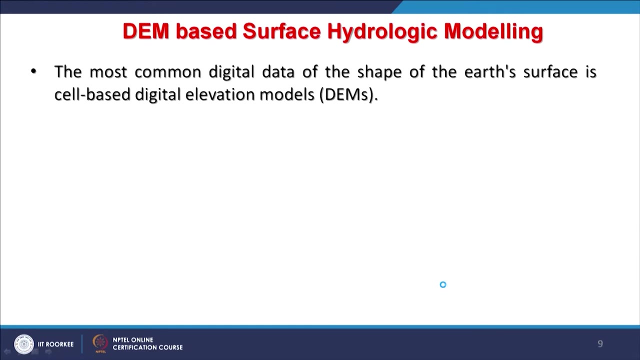 of your desired size. That would be decided based on the threshold value and that is basically the area which you give. So it is basically this. surface. hydrologic modelling, as you must have realized by now, is a sequential modelling, Means step by step. you can do it quite easily Now, as 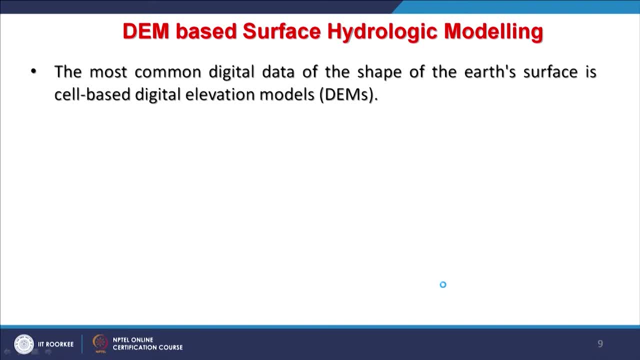 you know that the most common input is going to be a digital elevation model And we have already developed the understanding And this data is going to be a digital elevation model. So this is a sequential modelling And this data is going to be a digital elevation model. 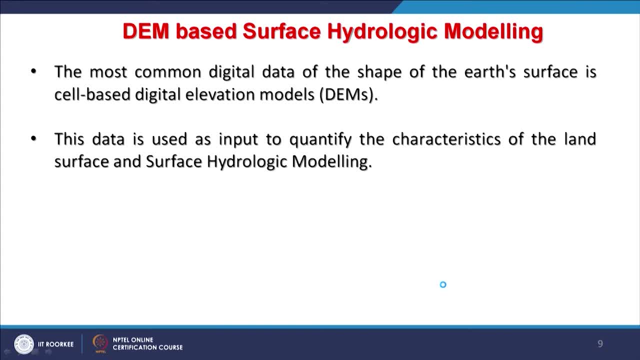 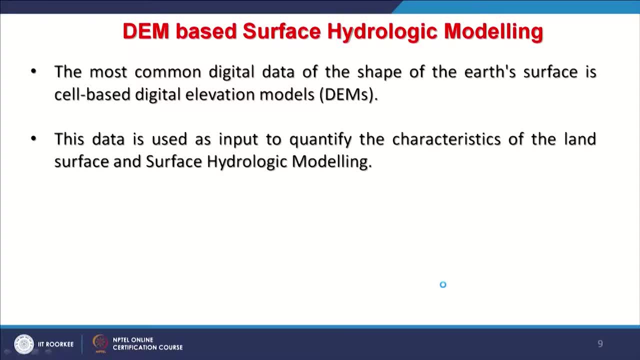 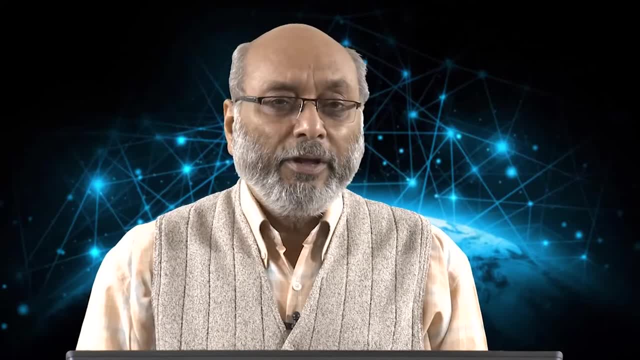 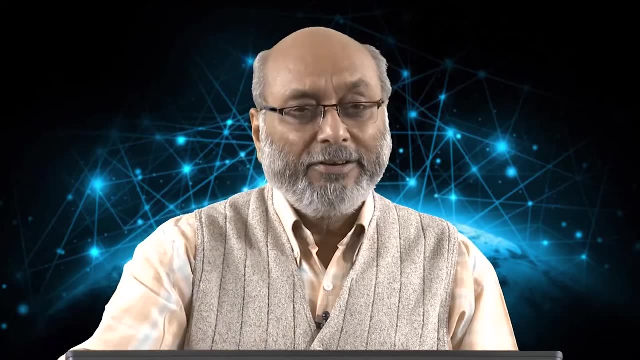 and that can be modelled through surface hydrologic modelling. Now, here the accuracy part will play a very important role. If your input digital elevation model is good- good means quality wise, accuracy wise- then obviously you would have a better results. This is true in all the cases. Now, other factors which will affect the quality: 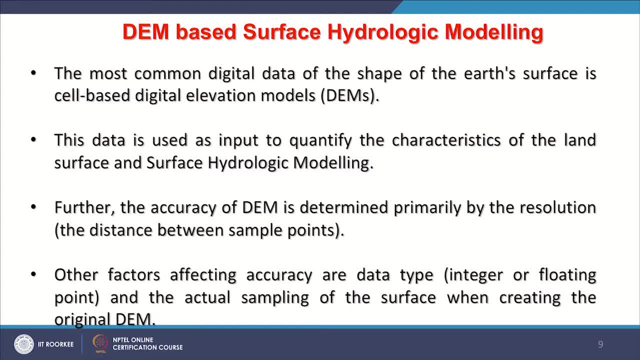 and accuracy are like, whether your input digital elevation model, because it is a grid, So you can have a cell value as integer or floating point. Floating point since it is having high precision and therefore the accuracy of your output is going to be very high. But 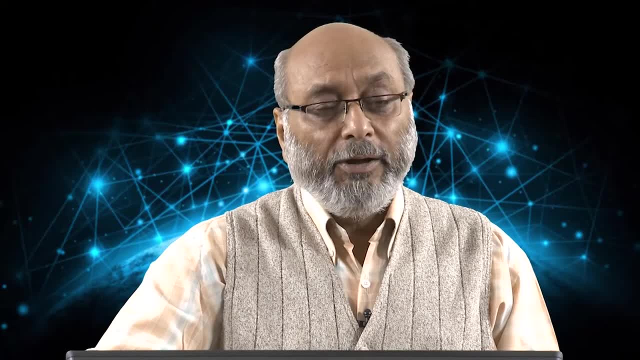 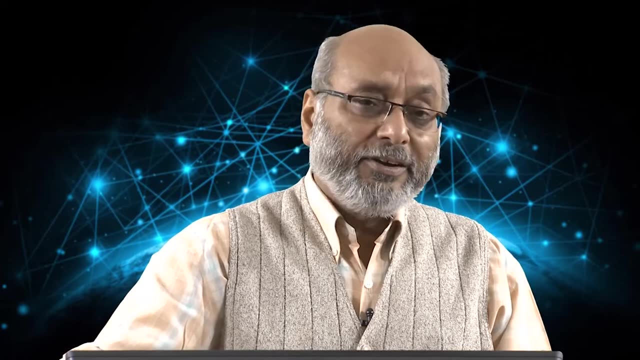 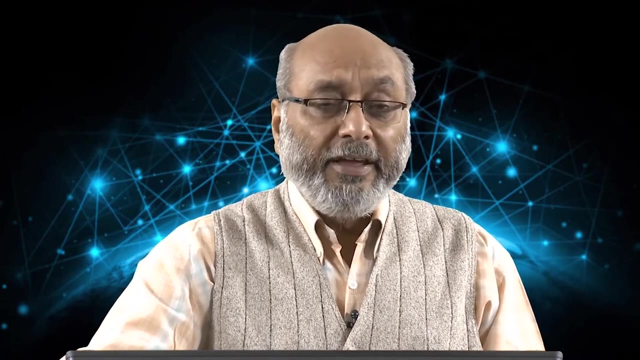 if you are having input points. input, you know, of digital elevation model- and cell values are integer. that means generally these are in meters, So you will have the least count is 1 meter and therefore the accuracy will affect. So this depends. If I am creating my own digital elevation model then I should keep the cell. 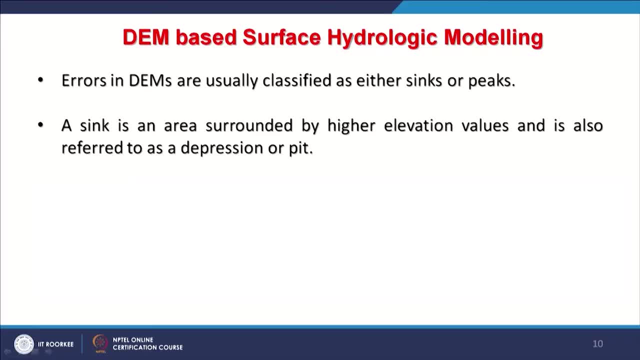 value as floating point or real numbers. Now, this is one type of error which can be rectified by first identifying sinks or peaks or depression and then filling them. So part of the problem is already solved and rest will depend. basically, the spatial resolution part. 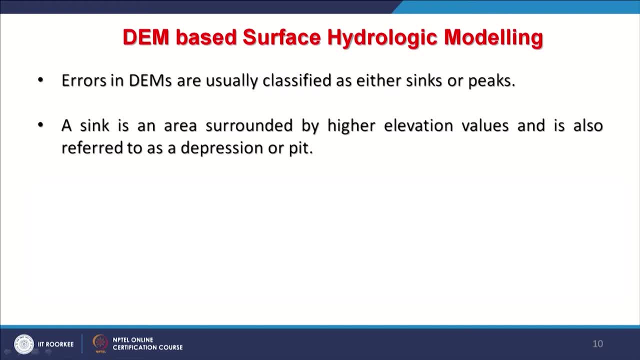 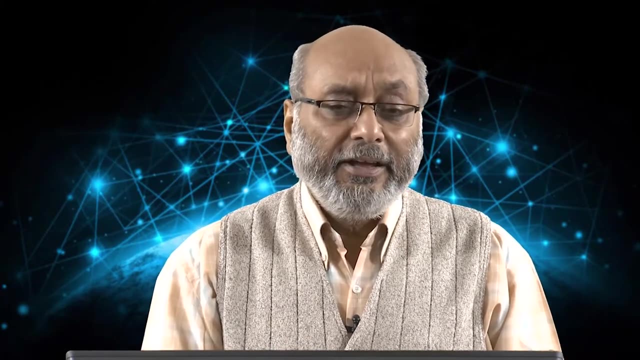 And a sink. as I have already explained, that sink, an area surrounded by higher elevation values And basically 3 by 3 kernel, is used to find out the pit or sinks depression and the centre cell is analyzed. If 8 surrounding cells are having higher value, then it is. the center cell. Then centre cell is identified as the sink and later on you fill it, because if it is not done, then it will develop its own internal drainage and then whatever the precipitation which is occurring will not come out, will not flow on surface as a surface. 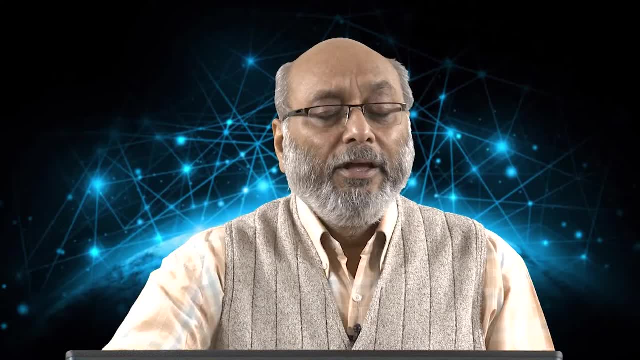 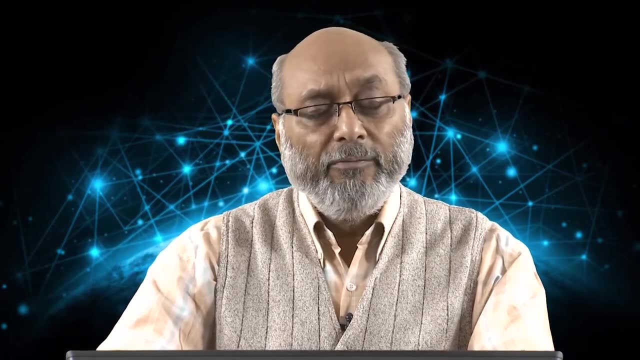 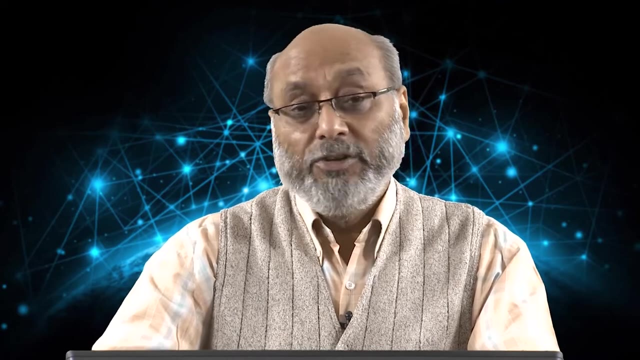 runoff and neither it will come out through the outlet. In many cases, you know, generally it will happen that whatever the precipitation is occurring will form a surface runoff and ultimately it will come out. But there are many natural conditions which may not happen like this. If it is a heavily forested water set there. will be completely lot of delay. It depends on what type of rocks are present, what type of structures- geological structures- are present and what type of soils are present, what type of vegetation is present, any human activities and some other like Whether it is a glaciated or not or a snow-covered or not, whether it is a karst area- Karst area. 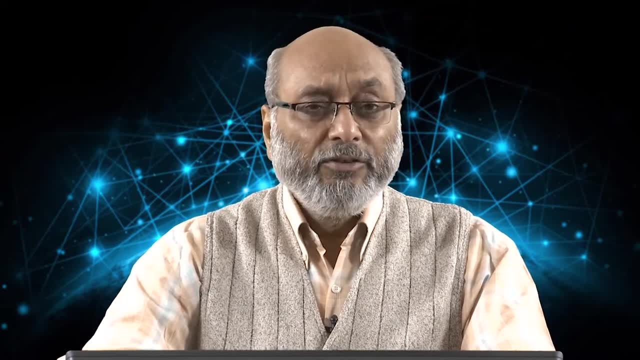 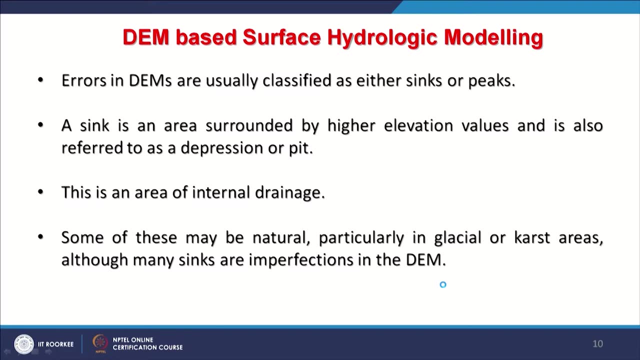 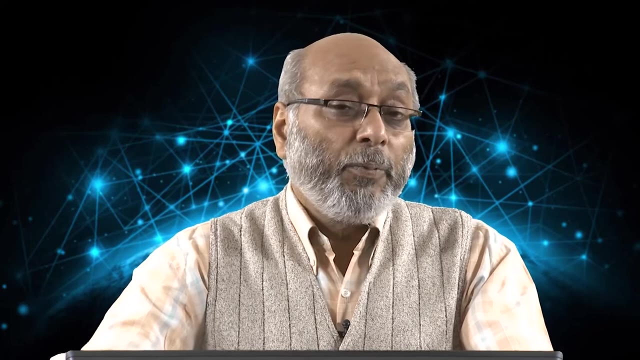 means terrain of limestone terrain, Because limestone terrain is generally having internal drainage. So on surface you do not see the drainage but internal drainage. So the surface hydrologic modelling may not predict as you wish to have because it will not follow that. 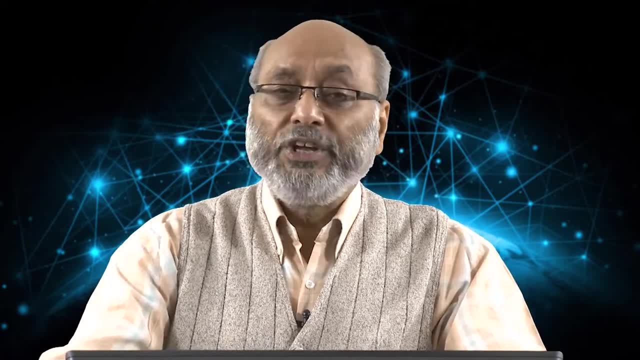 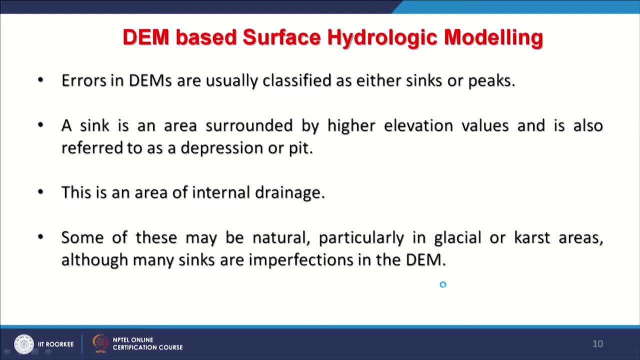 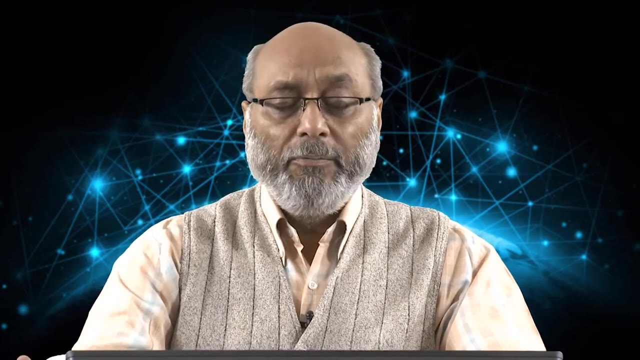 assumption. The assumption is that even a single drop of water, if it falls on the surface in a watershed, it has to come out through the outlet. So in many conditions this assumption is not fulfilled, But nonetheless, in many-2 conditions it is fulfilled, Even if it is not being fulfilled. 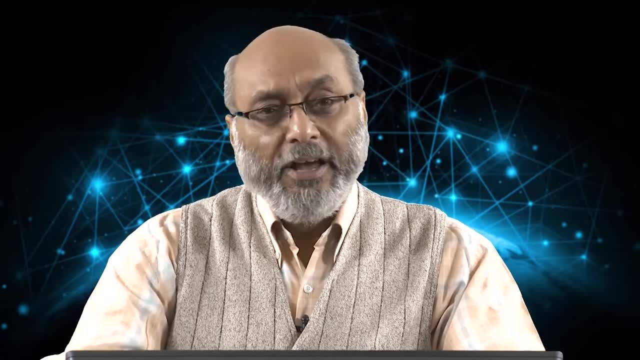 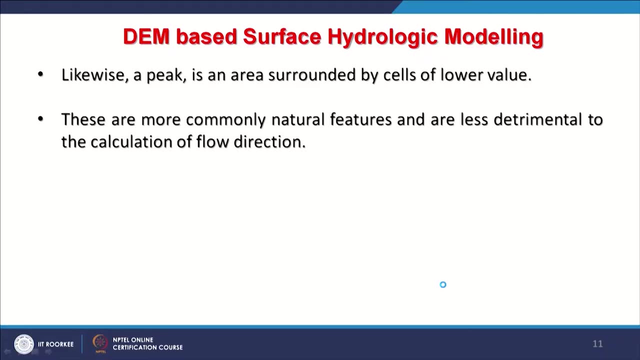 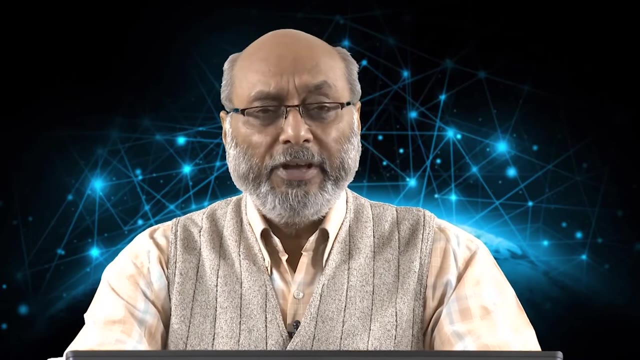 still, we can exploit and see how it affects the groundwater, which we will discuss little later. Similarly, when we identify sinks, we also identify peaks, but peaks will not affect much in that way. But nonetheless, in that process everything is identified, Then it is made. 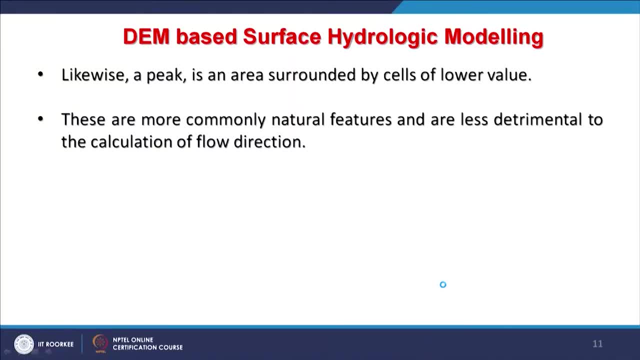 sure that whatever the water which is dropping on the surface in a watershed has to come out of outlet. Now this flow direction, that is, these are the more commonly natural features And the area less determined to calculation of the flow direction And errors, such as. 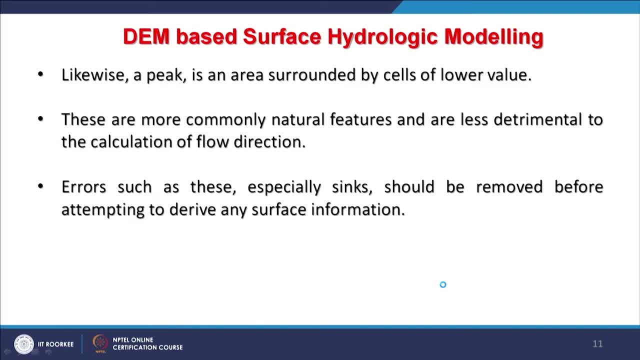 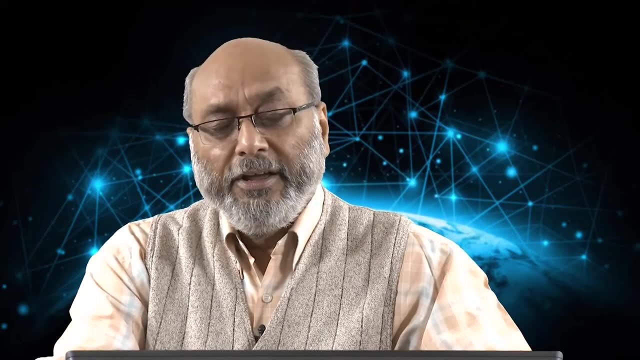 of these, like sinks or peaks, should be removed before tending a device to derive a surface information or before we go for next step in surface hydrologic modelling. Because water has to flow. that is the assumption. If it is just in one cell, it becomes a step in. 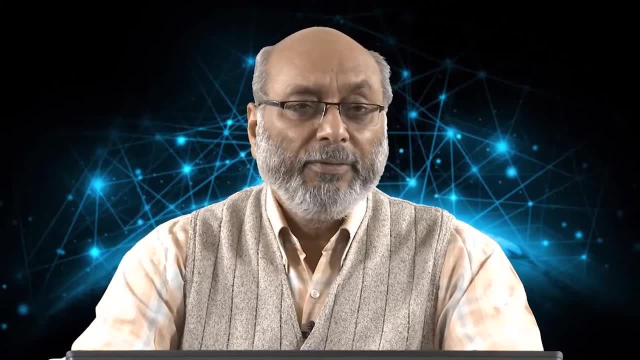 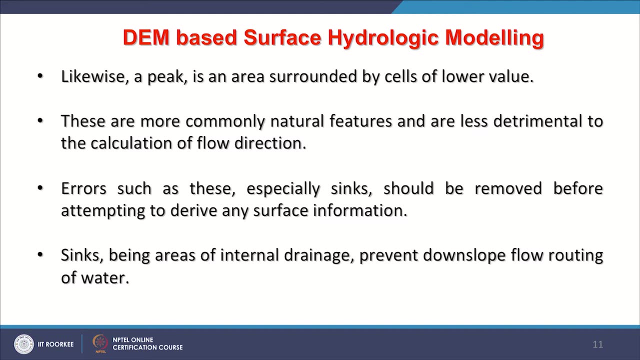 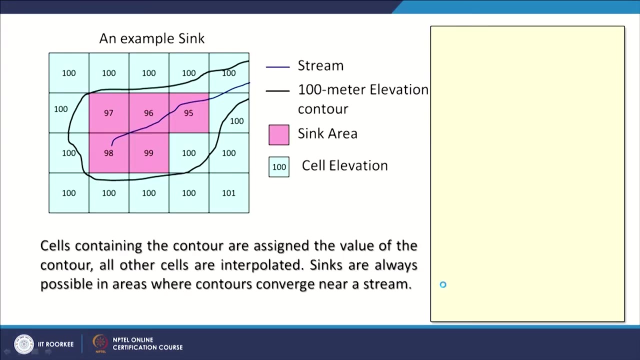 it becomes stagnated, then it becomes a problem. So sinks may be areas of internal drainage, like I have said in case of limestone terrain, or can prevent down slope flow routing of water. Now here is the example. There may be a single cell representing a sink or a depression, having multiple cells In this. 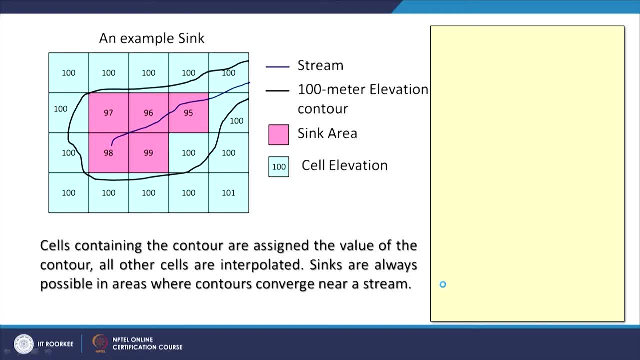 example, there are 5 cells which are having depression. So all surrounding cells here are having higher values than these pink coloured cells. So we identify them as a sink And rest. as you can see, the contour lines are also shown here. These are not watershed boundary, Mind it. This is contour line and stream network. 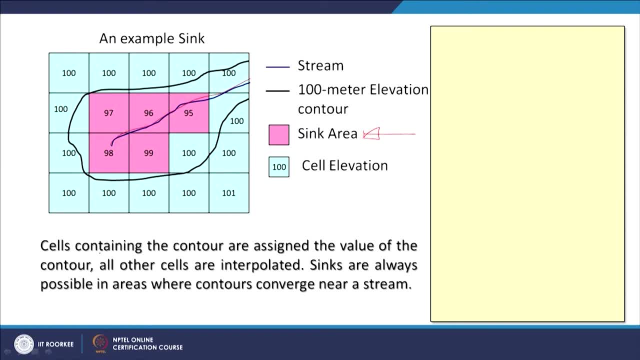 also shown here. So basically, cell containing the contour line and assign the value of the contour, The entire fringe cells are interpolated in a manner that no sink will be there. So sinks are always possible in areas where contours coverage near a stream. 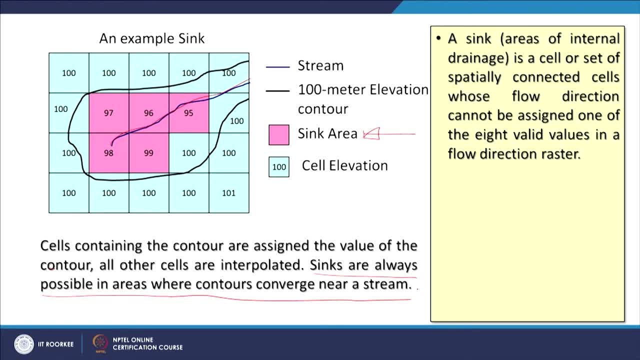 Now sink or areas of internal drainage, is a cell or set of cells which are spatially connected cells and whose flow direction cannot be assigned. So for flow and for that kind that purpose also, we have to do that part. So generally in practice, what we do that once we take the digital elevation model, 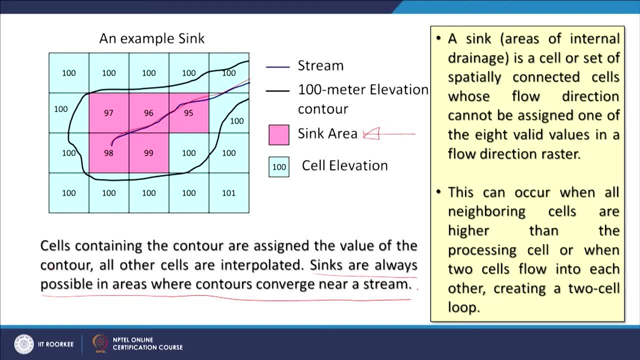 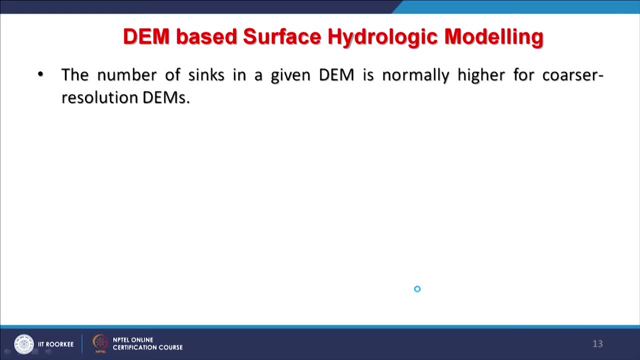 first we do this sink identification and filling, Then we go for flow direction and flow accumulation and other derivatives. That is always because if there is error, let us remove at the very first stage. Now the number of sinks in a given digital elevation model is normally higher for coarser. 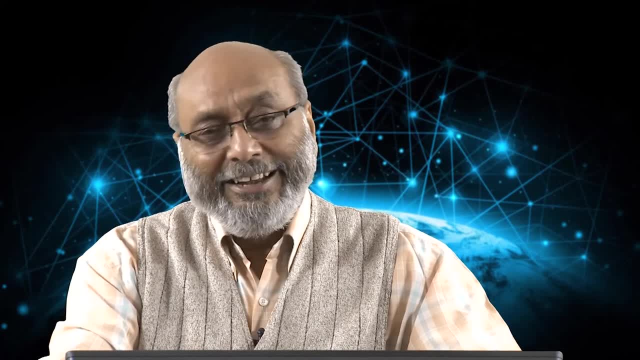 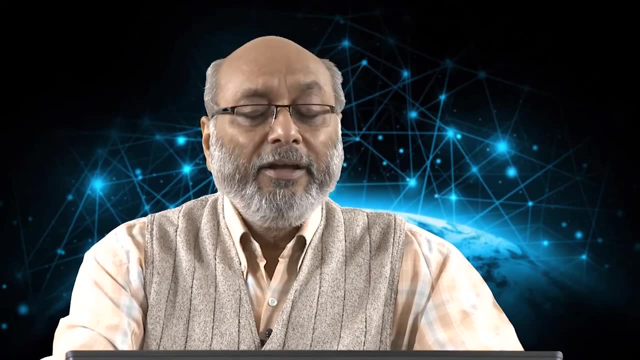 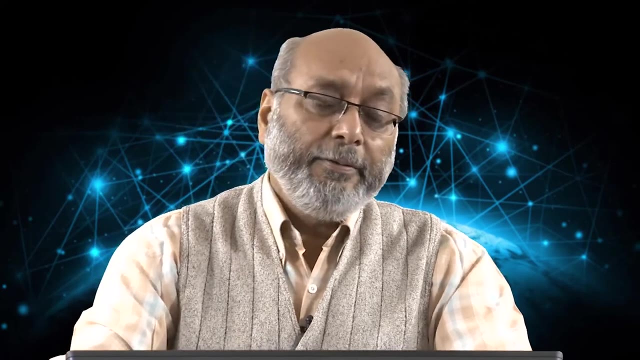 resolutionDM. So in a relatively, if you are having a coarse resolution digital elevation model, the area which will be covered by these sinks is going to be very high. In a high spatial resolution digital elevation model it is just the reverse case. So in this case, 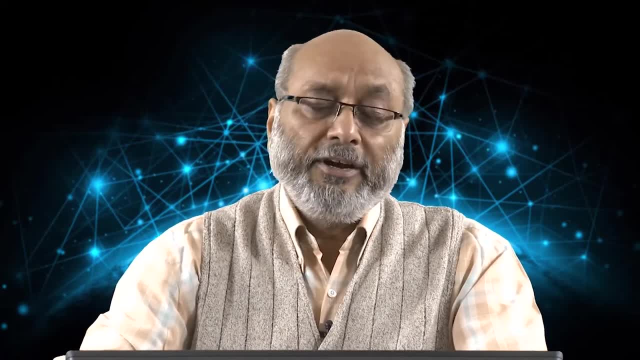 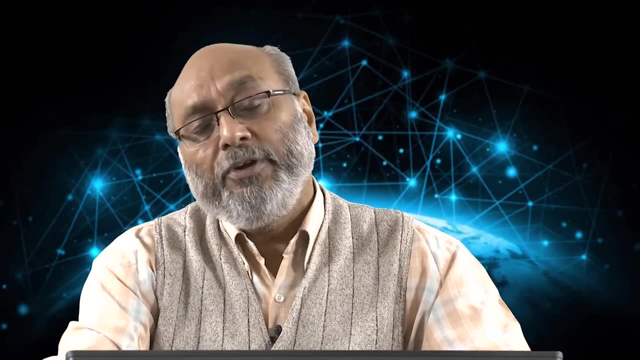 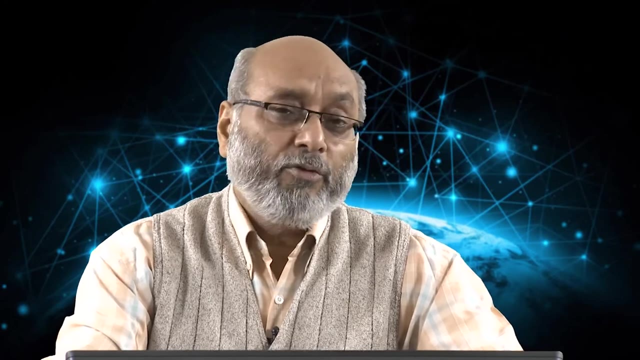 for surface-level logic modelling. if choice is there, it is always better to go for relatively high spatial resolution digital elevation model. But, as when we have been discussing the quality of a digital elevation model, we also discussed that high spatial resolution does not always mean a high, accurate digital elevation model. 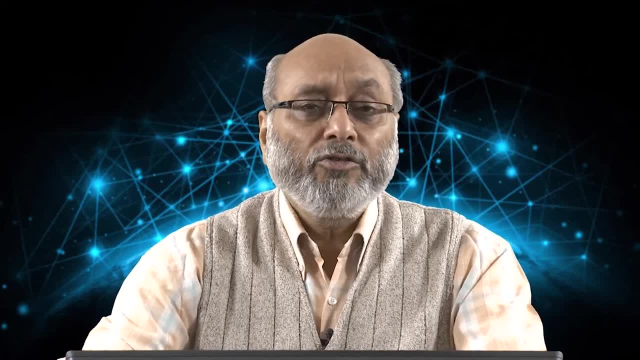 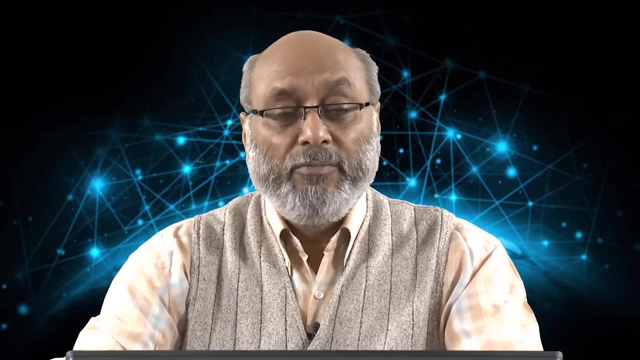 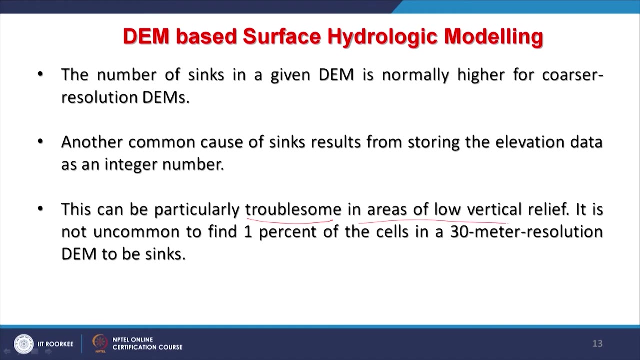 So that one has to also remember. Another common cause of sinks in a digital elevation model results from storing the elevation data as an integer number, not as a real number, And this can be more troublesome in areas of low vertical relief, That means the area which do not have much undulations, and you may have problem. 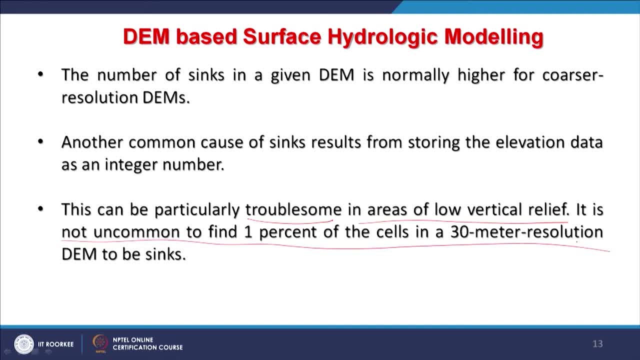 Now, it is not uncommon to find 1% of cells in a 30-meter spatial resolution DEM to be sinks. But 1% is nothing in that sense. Now this percentage can increase by multi-folds if we are having a 90-meter, that 3 arc. second, 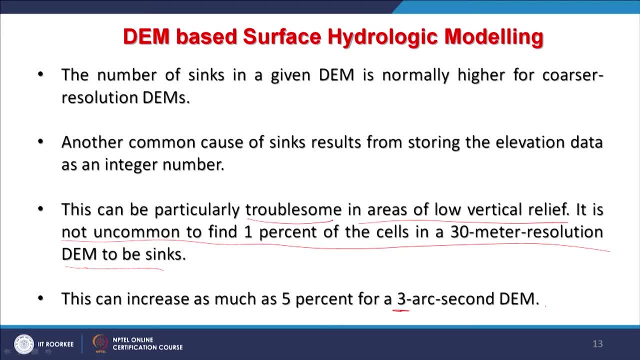 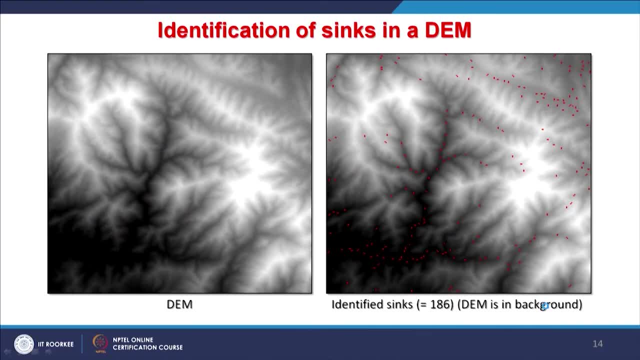 equal to 90-meter roughly, and 1 arc second equal to 30-meter, So 3 arc second digital elevation model. Now I am having an example on the same digital elevation model which we have been using throughout this course. So this is the DEM. 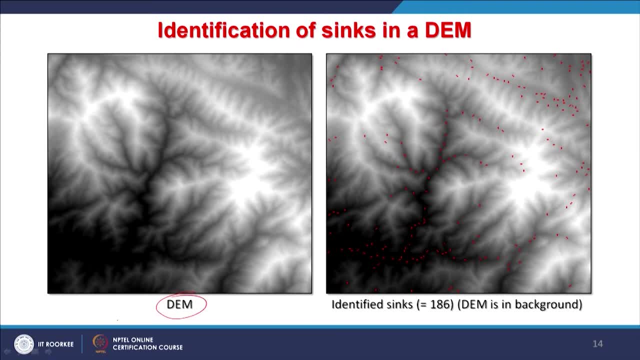 And when DEM is subjected for identification of sinks. You can see these red dots. these are sinks have been identified. Some are single cells, some are having set of cells, So identified sinks. here its total number is 186, whereas digital elevation model total. 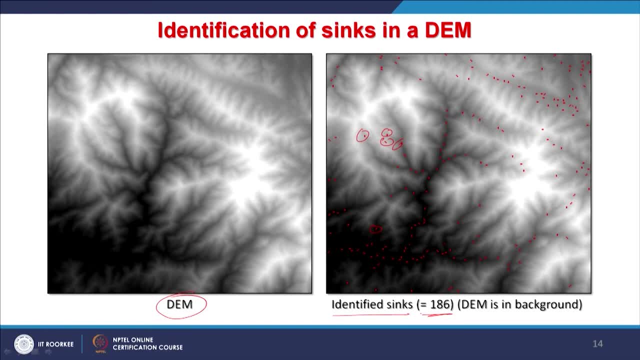 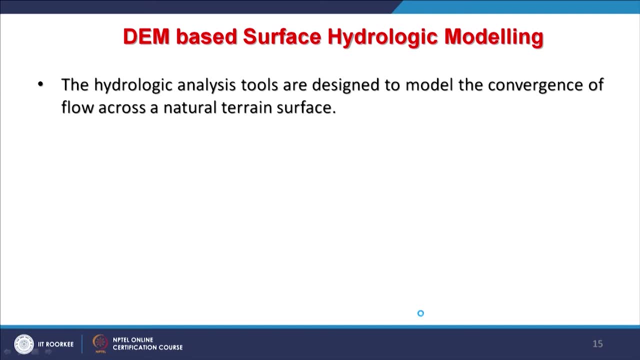 number of cells are, you know, 99 times more than this, roughly Now. once we have filled the sinks, then we come to the next step, That is, your flow accumulation or, before that, flow direction. So these hydrologic modelling tools, or hydrologic analysis tools, basically have been designed. 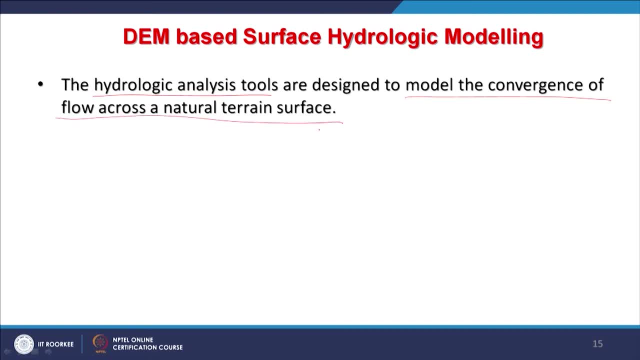 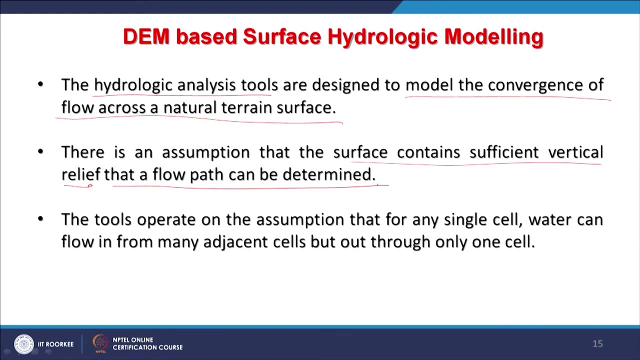 to model the convergence of flow across a natural drainage system or terrain, And the assumption, which I have already mentioned, is that the surface contains sufficient vertical relief That a flow path can be determined, That whatever is falling in form of precipitation has to flow and it will create own path through. 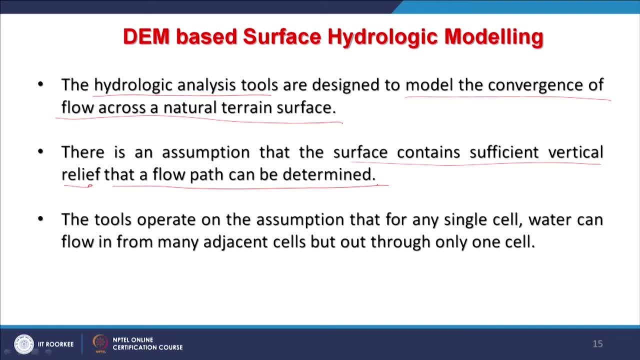 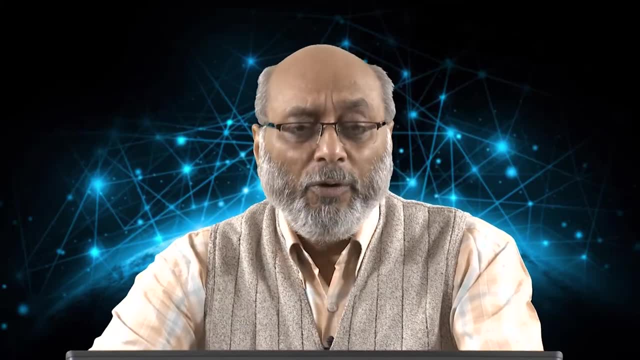 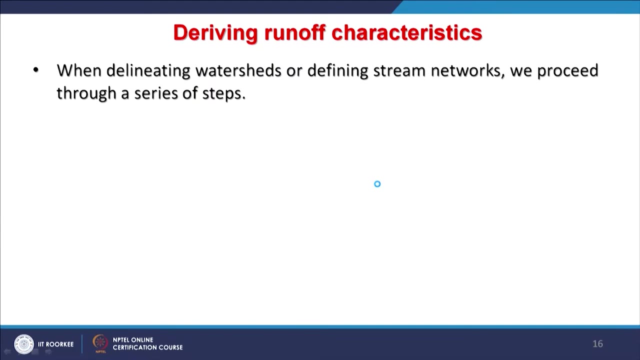 a drainage network in form of drainage network, And these software tools operate on the assumption that any single cell water can flow in from many adjacent cells but out through only one cell. Now, when we go for the delineation? Okay, So for the delineation of water cells using surface hydrologic modelling or defining stream, 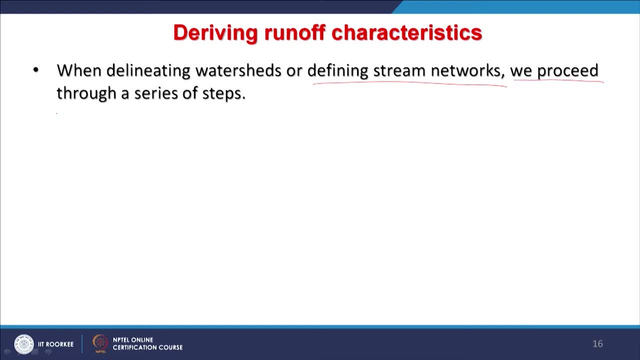 network. we process through a series of steps. That is why I said earlier that surface hydrologic modelling is a sequential modelling. So series of steps, 1 by 1, we will go. Some steps are required while others are optional, depending on the characteristics of the input. 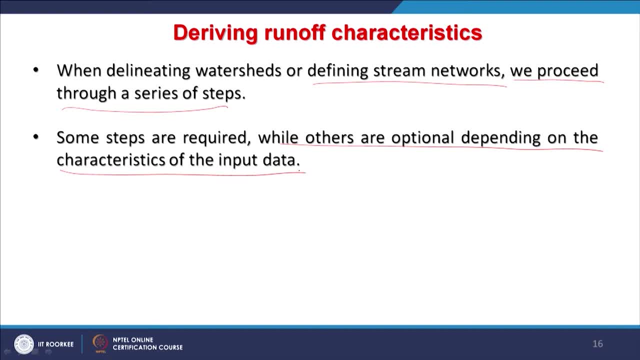 data And whether we really require those outputs. Okay, Whether we require those outputs or not, And flow across a surface will always be in the steepest down slope direction. So whichever the cell is having more difference in terms of elevation, there the water will. 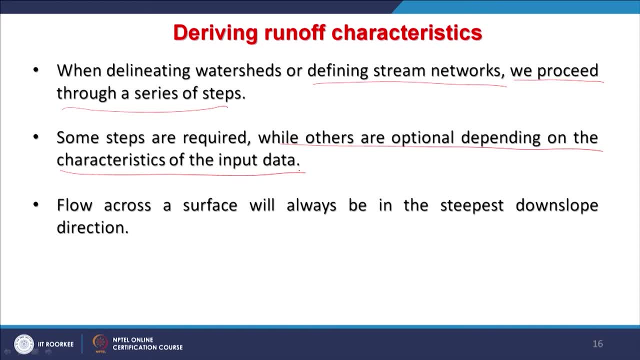 flow from the centre cell if we think in terms of that 3 by 3 kernel. Once the direction of flow is decided out of each cell in the known, it is possible to determine which and how many cells flow into in the known. Okay, 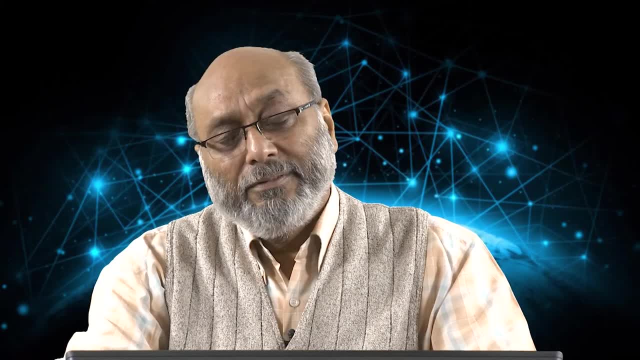 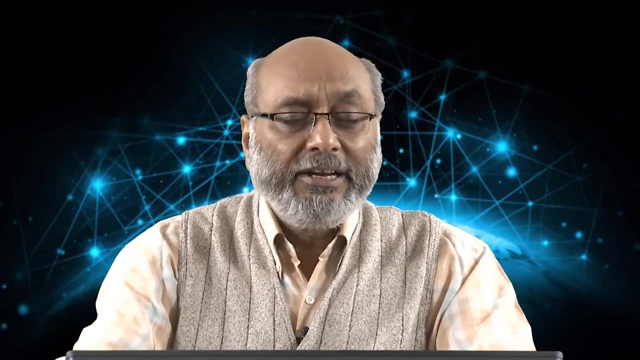 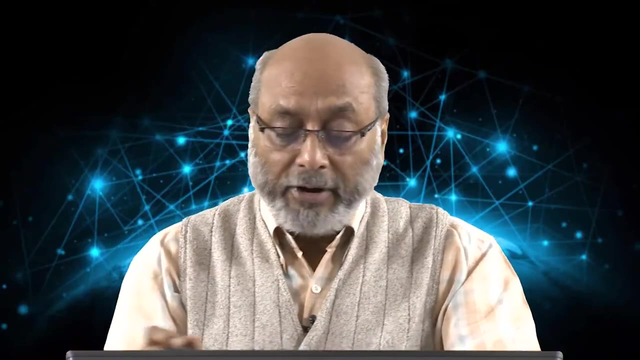 Thank you. So each cell has to flow out, But how many cells will flow out in one cell? that will be also determined through flow direction, And the information then can be used to define watershed boundaries and stream network. So these are two derivatives through the surface hydrologic modelling. 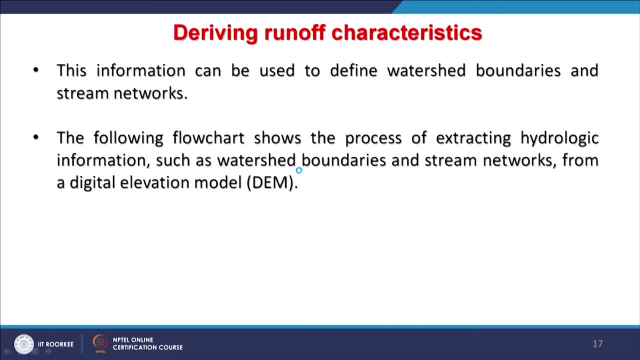 Very popular one, or you can say first order derivatives. Okay, So the flow chart which we have discussed again I am going to show, which shows the process of extracting hydrologic information, such as watershed boundaries, stream network, through using a digital elevation model. 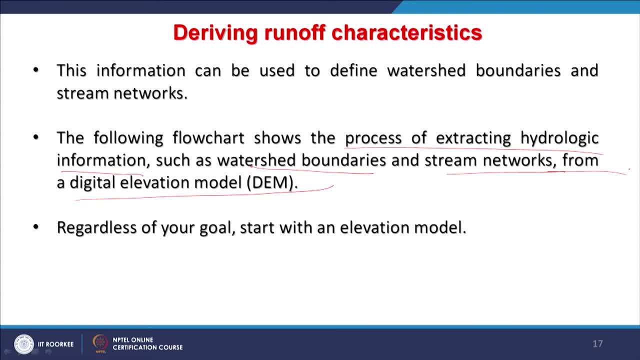 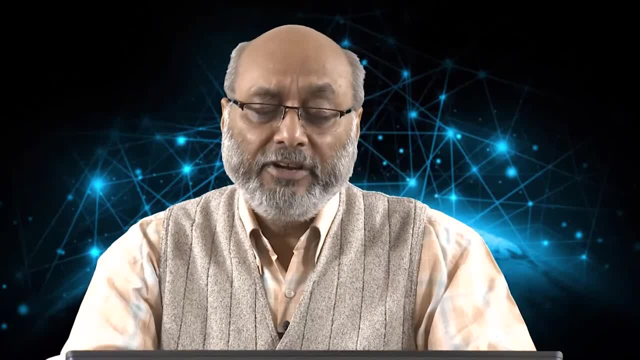 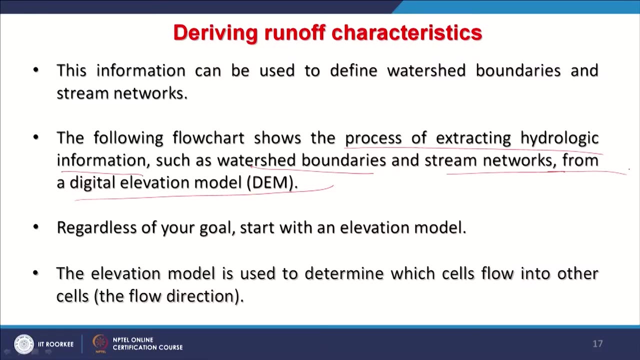 Whatever the purpose of using this surface hydrologic modelling, the start point has to be always as a digital elevation model and identification of sinks. So elevation model or digital DEMs are used to determine which cells flow into other cells, that is, flow direction. 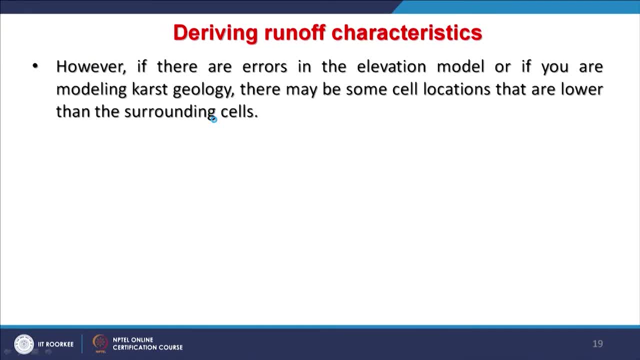 This is the flow direction which I am talking Now. if there are errors in the elevation model, which we have also touched upon this issue- then, like maybe a limestone terrain, a karst topography or karst geology, there may be some cells, locations that are lower than the sink. 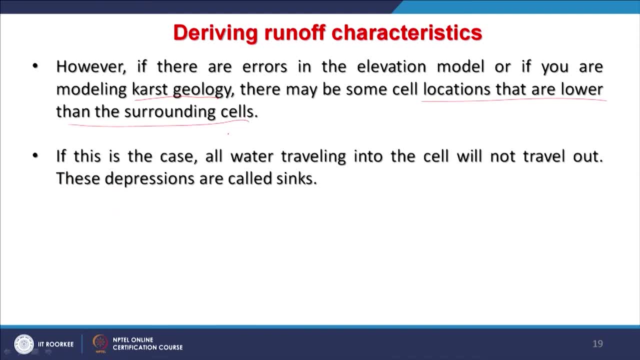 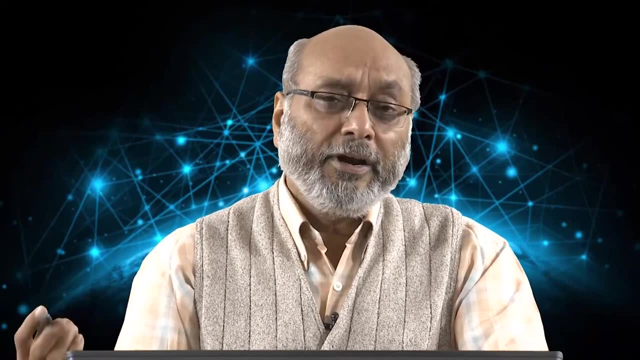 Okay, But in the surrounding cells an internal flow might be there. So there is a limitation of surface hydrologic modelling. that means in those conditions the surface hydrologic modelling will fail because the assumption here that each and single drop of water has to flow as a surface runoff and has to come out of a watershed. 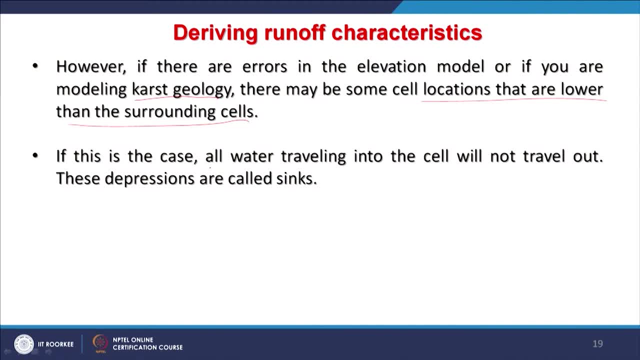 And if, in case of karst topography, all water travelling onto the cell will not travel out, And if that does not travel out, then this surface hydrologic modelling will not work. So our tools, the surface hydrologic modelling tools which are available in most of the popular 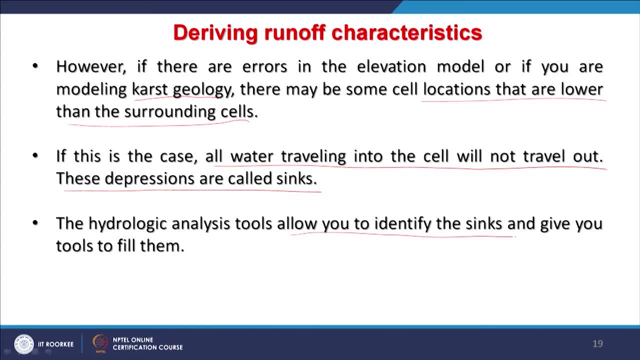 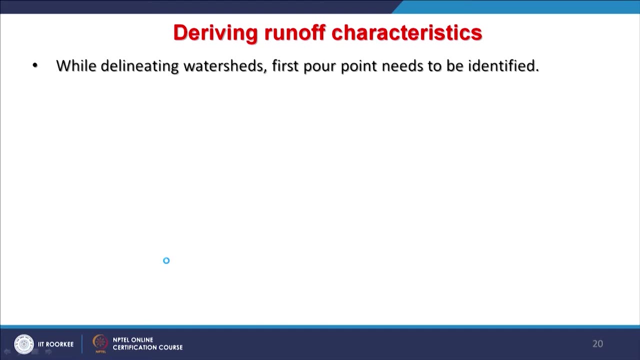 GIS softwares will allow to identify sinks and give you tools to fill them. I have shown the example also And ultimately then you will have a depression: less elevation for further processing. Now one of the outputs or derivatives of sinks, The derivatives of surface hydrologic modelling using a digital elevation model, is delineating: 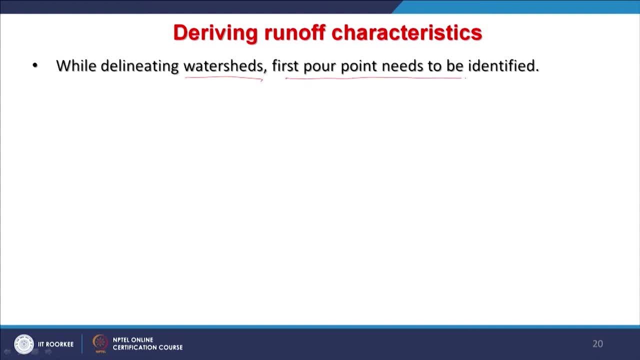 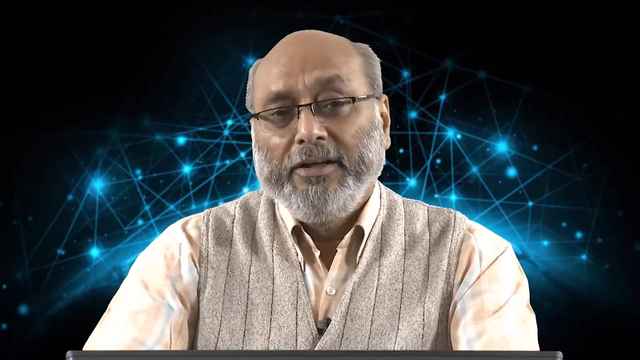 a watershed, That is the first pore point needs to be identified for that, And usually these locations, the pore points, outlets- are the mouth of the stream or other hydrologic points of interest, such as gauging stations. So in the beginning of this discussion, when we have been discussing about this part, we 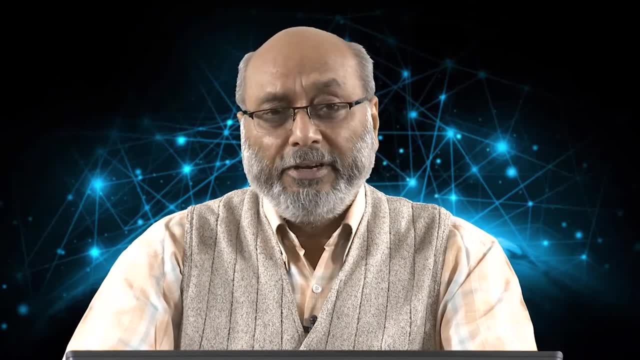 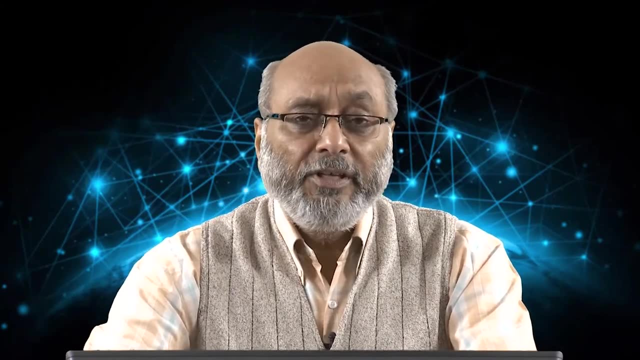 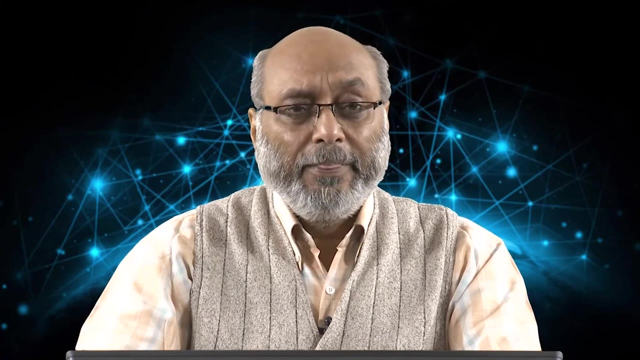 have already discussed the terms which we are going to use about watershed there And in this surface hydrologic modelling. once the pore point has been identified, then the system will automatically delineate the watershed. Of course, stream network and other things will also be done. 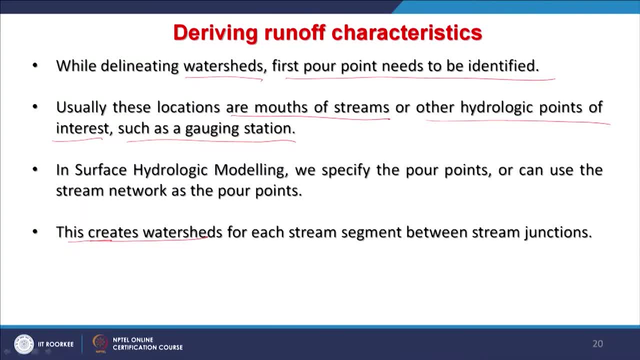 And this creates the watershed. once you have selected a pore point for each stream segment- That means sub-sub-watersheds- you can go to a single stream between the stream junctions And to create the stream network. the first flow accumulation for each location is calculated. 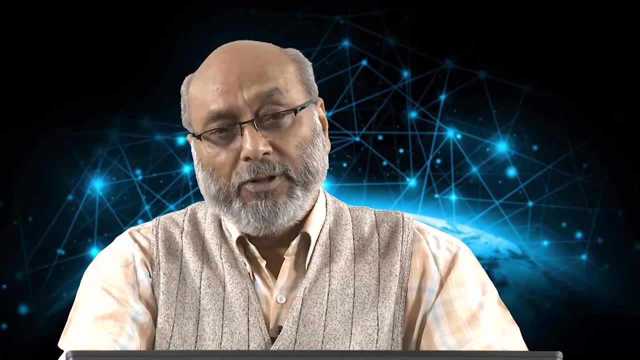 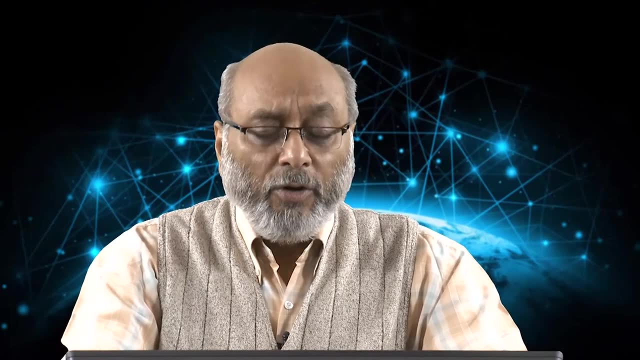 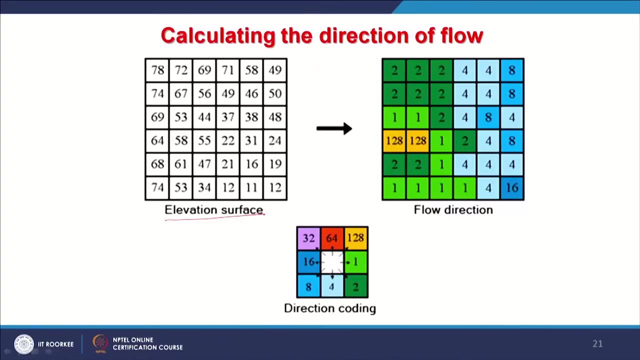 So this is virtually the fourth step. The first step is to identification of sinks: filling of sinks, flow direction. now, flow accumulation. Now, in case of flow direction, how it will look in terms of digital values. So here we are having input, digital elevation model. 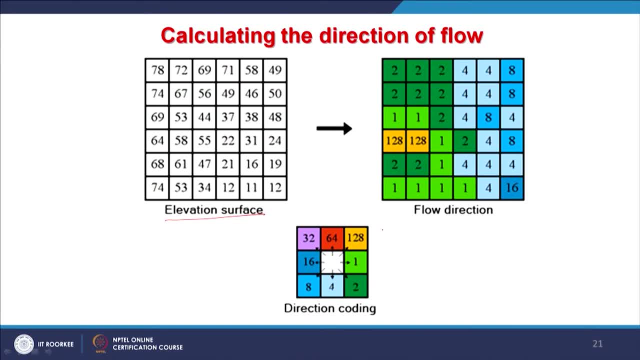 Here we are having this 3 by 3 kernel and a coding system, So for each direction we are having code 1.. This is though it is a number, but it is a code. That means we will not do any arithmetic operations over these codes. 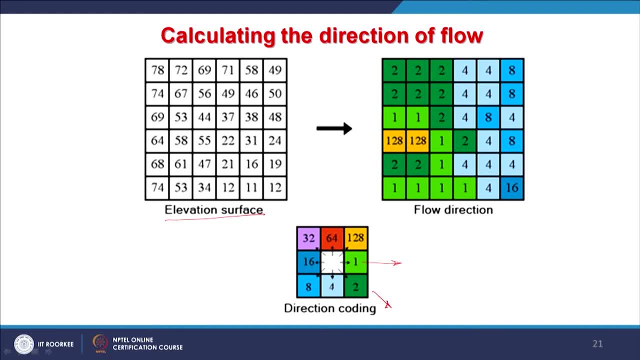 For the south-east direction, the code is 2.. For south direction code is 4.. And for south-west direction, 8 and likewise. So when this 3 by 3 kernel moves all along over a digital elevation model, this is how. 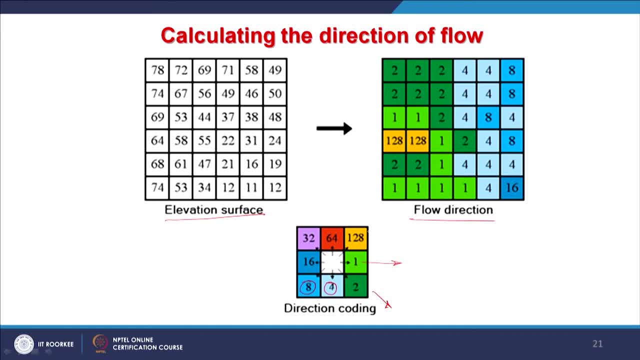 it will have a flow direction. So 128 means it is flowing in the north-east direction. Now let us see for these cells that here this is 58 and this is 61 and 68.. So 68 is very high among these. 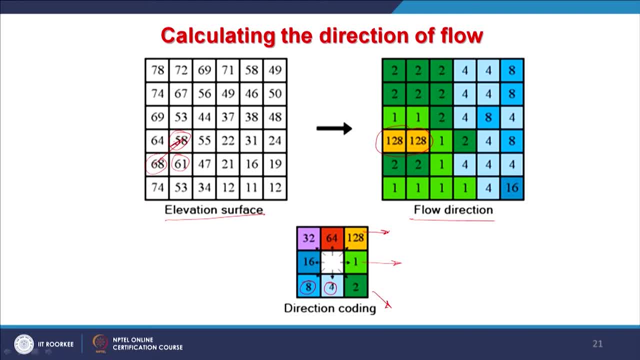 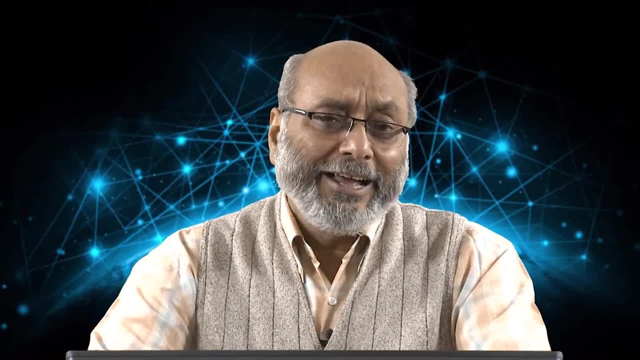 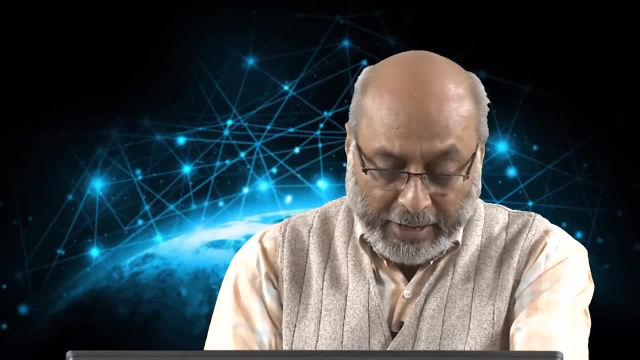 So this will flow in this direction, that is, in the north-east direction. Similarly we can understand the other So flow direction. while calculating we use this concept of 3 by 3 kernel using codes. So flow direction: a conclusively definite line or course in which something is issuing. 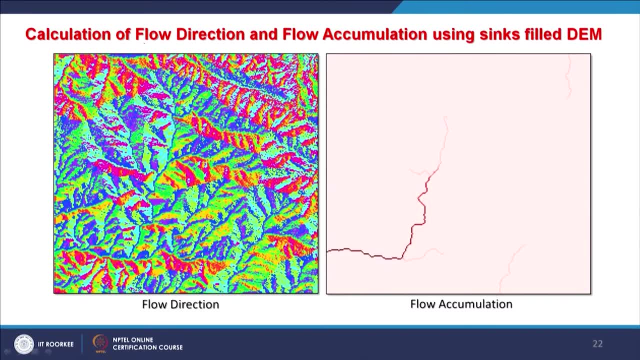 or moving into a stream. On the left side you are seeing a flow direction derivative through surface hydrology modelling, And on the right side you are seeing flow accumulation, Though here you may feel that only few lines in form of drainage are visible. rest is not. 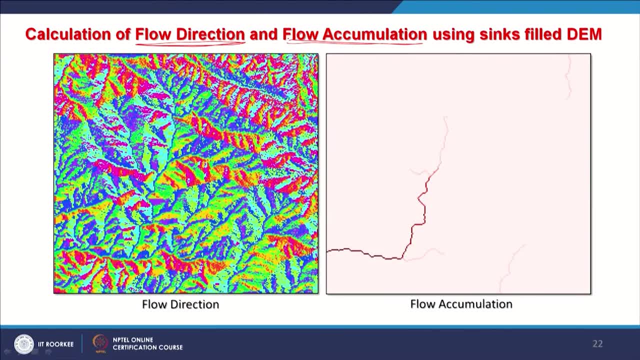 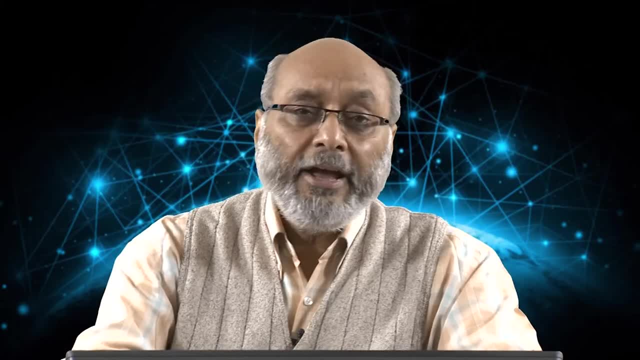 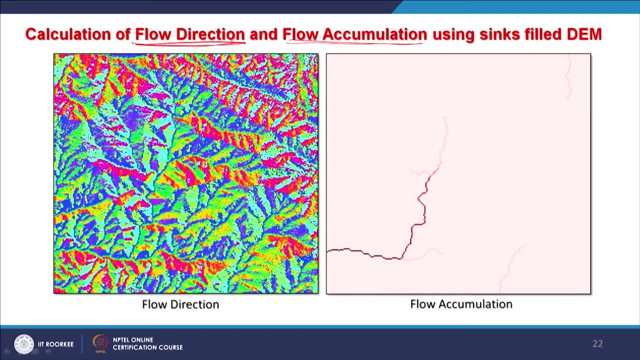 there, But each cell is having a value which you can check while zoom it and using identification tool. So that is why I said earlier also, Flow direction is more or less like an aspect map, very close to that concept, But the coding part is little different because these numbers are required, not the north-east. 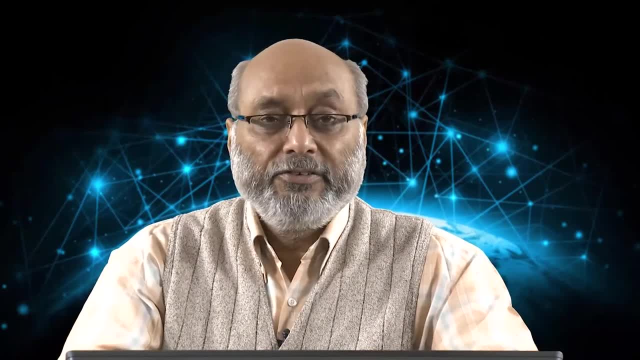 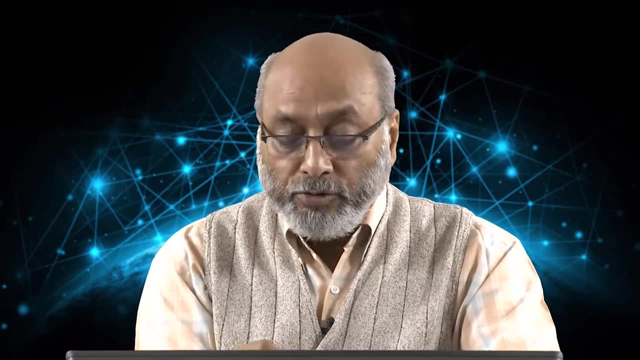 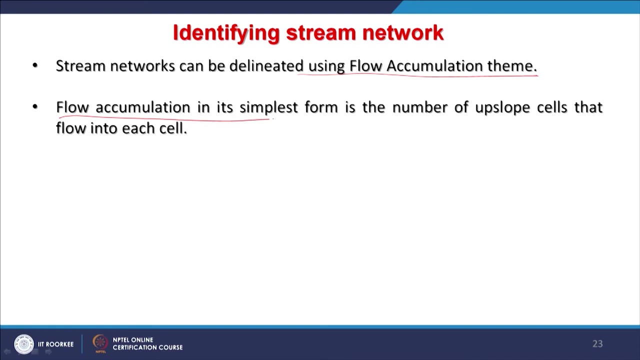 south-west. These numbers are required in different calculations, So that is why the coding system has been adopted for flow direction. Now stream network can be delineated using flow accumulation theme, which is the fourth derivative. Flow accumulation is its simplest form. we can say that the number of upslope cells that 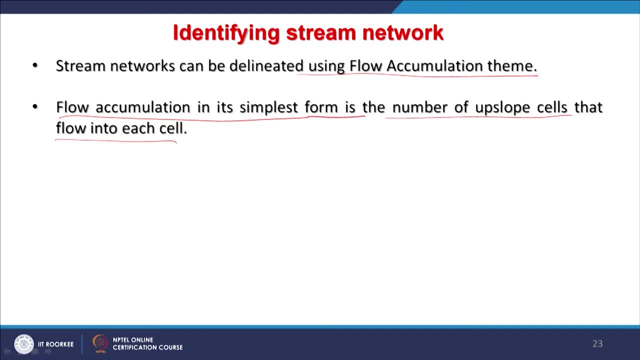 flow into each cell, because drainage network will be decided, stream network will be decided based on the number of upslope cells And by applying a threshold value, that if 100 cells or 1000 cells are flowing at an outlet. that becomes my pore point. 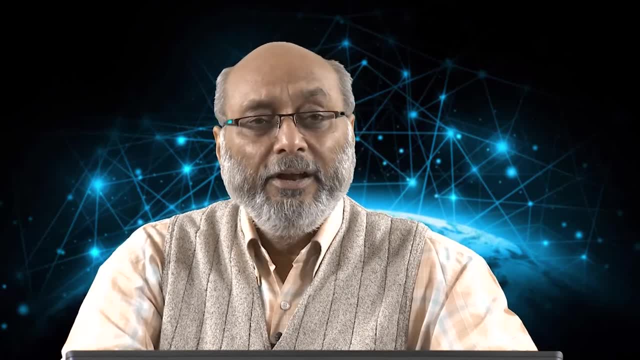 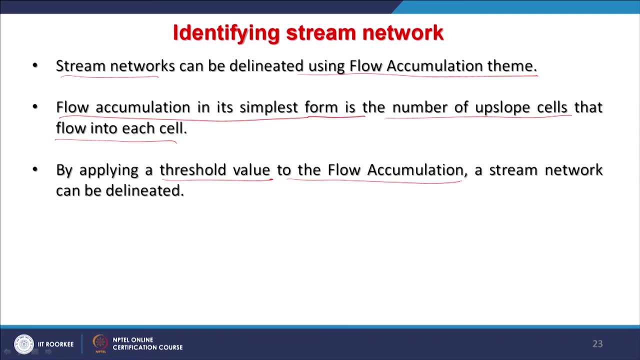 And then water set boundary or drainage network can be determined. So this is what we can do. Okay, So by applying a threshold value in terms of number of cells to the flow accumulation, output or theme, a stream network or a water set boundary, boundaries can be calculated. 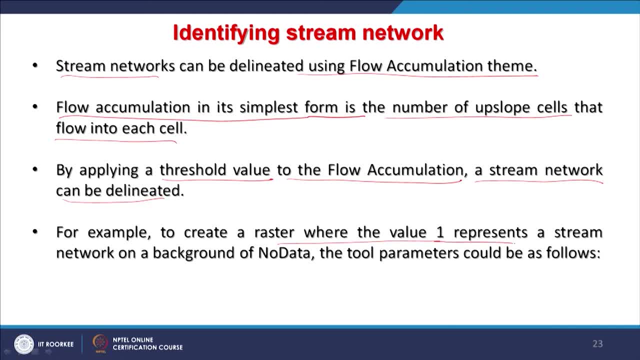 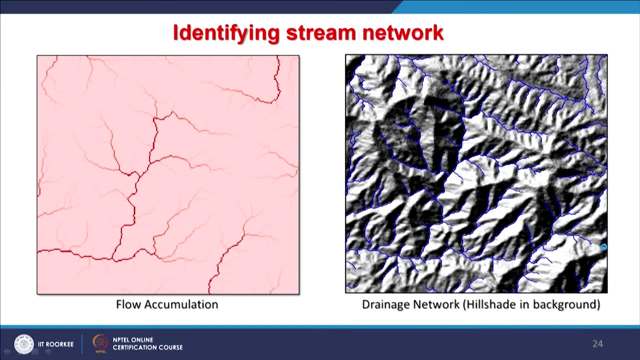 And, for example, to create a raster where the value of 1 represent a stream network on the background of no data, and the tool parameters could be as follows: that, for example, threshold value equal to or more than 100 cells. This is what it has been done. 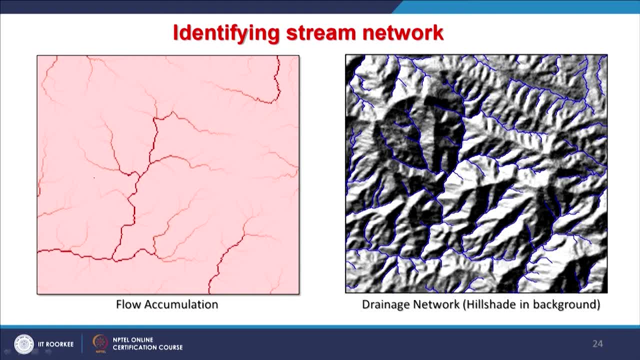 Once it is applied. drainage network, now flow accumulation. you are seeing lot of drainage there And using that I can identify these drainage. So from raster I can convert into the vector So the blue lines which you are seeing and in the background you are seeing a shaded 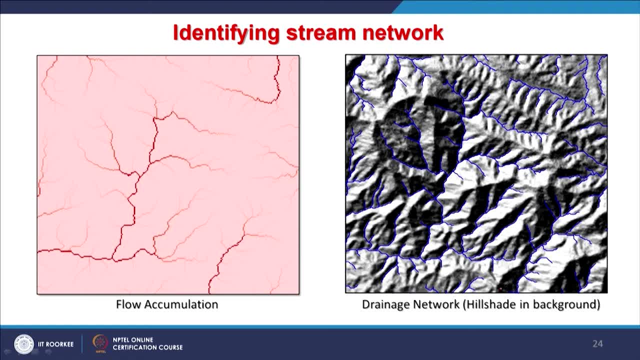 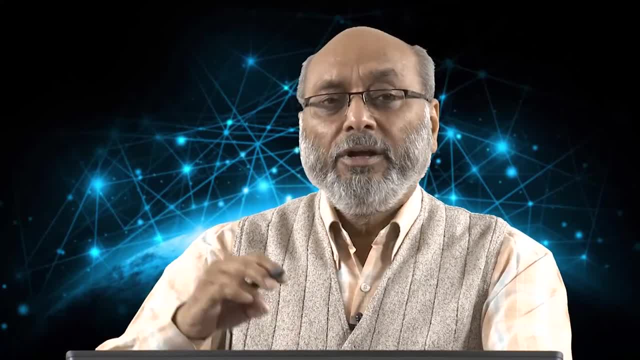 relief model, which is again derivative digital elevation model. These blue lines are the digital relief model. So this is the digital relief model. These blue lines are vector drainage network which has been derived through the same DEM, through this surface hydrologic modelling, where the threshold value was kept at 100.. 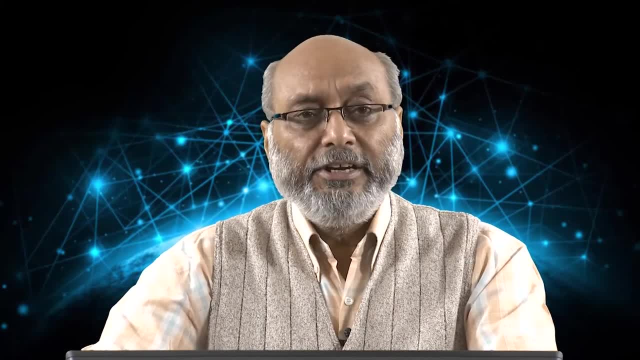 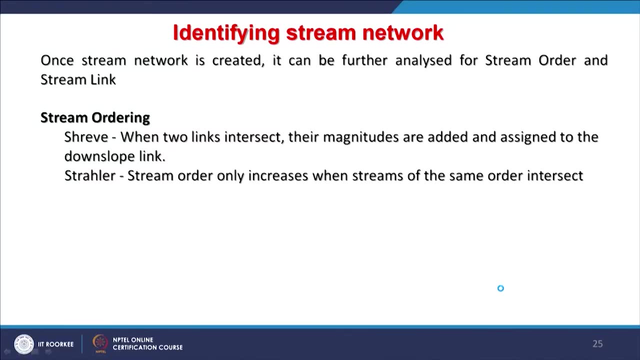 Now, once the stream is created, stream network is created, it can further be analyzed for stream order and stream links, which are again useful in some other modelling. So stream ordering, stream methods and stellar methods, So two methods are well established. 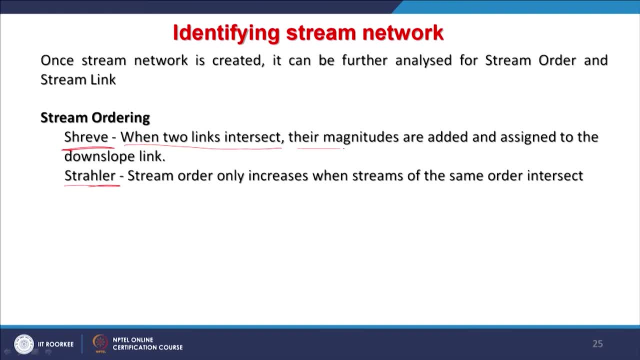 In first method. when the two links intersect, their magnitudes are added and assigned to the downslope link, like here. So order 1, first order, first order. when these two adds up, it becomes the second order. When second order and first order becomes again, it goes for the first method. 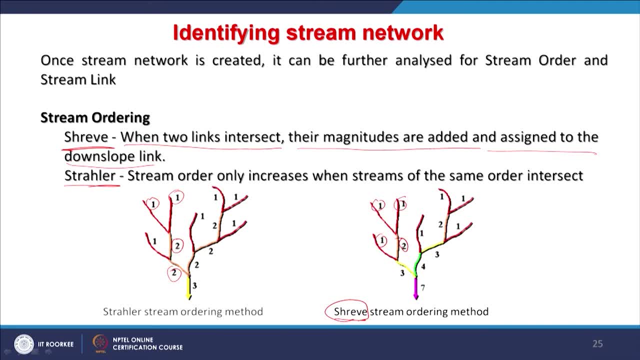 So, first order, first order, It becomes second order, First order and second order, it becomes third order. This is the stream method, the first one, And the second one is the stellar method, where the first order, first order, of course, becomes. 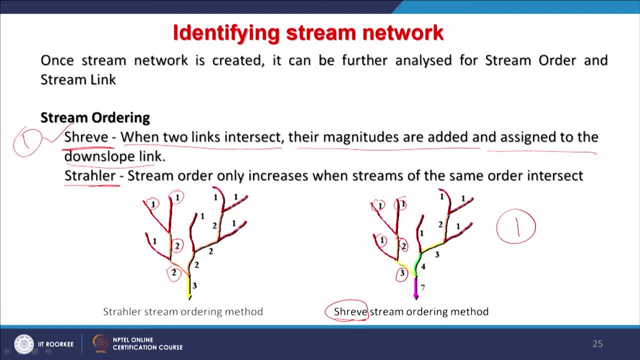 second order, But second order and first order will remain second order, And when two second order streams meets, then it becomes third order, not the fourth order as in case of here. So there is only little difference. but the stream order is very simple and this is most. 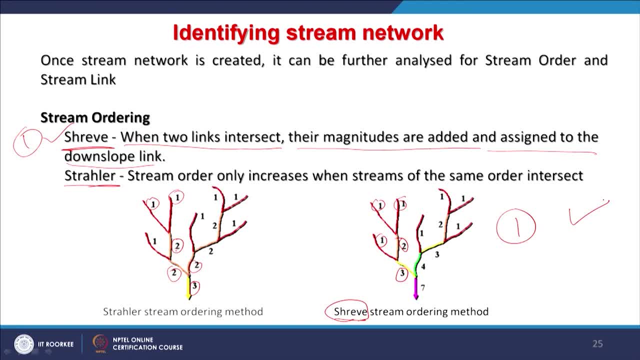 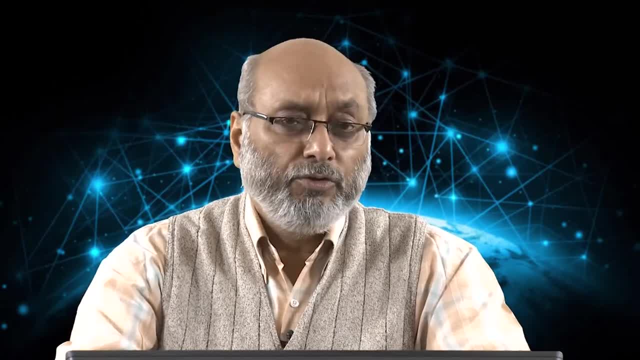 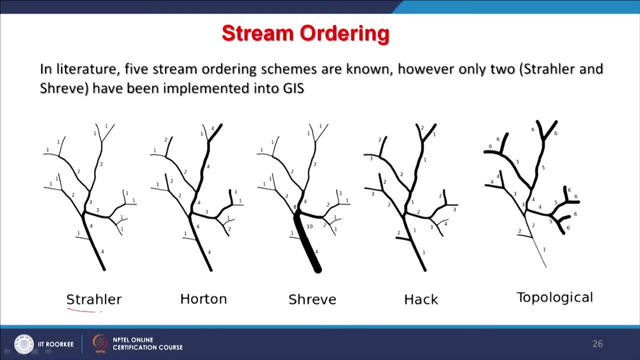 popular. However, in good standard GIS softwares, both stream schemes- ordering schemes have been implemented, So whichever you like most, you can use them Now. stream ordering: as you can see, there are other methods also apart from the stellar. 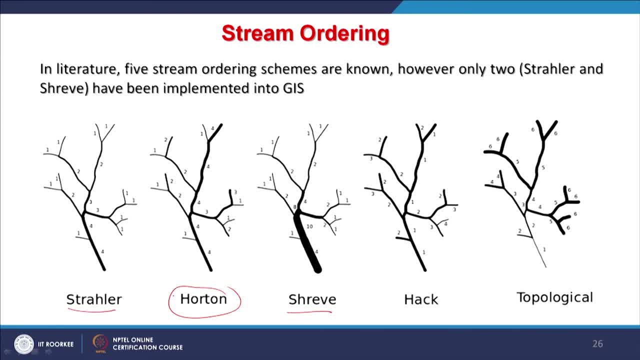 and stream. there are methods. Horton Horton has worked lot on in this because you have also seen the new algorithms for slopes aspect and other things: Hack method And, of course, a topological method that is based on the topology. So in literature you may find 5 stream ordering schemes are known. 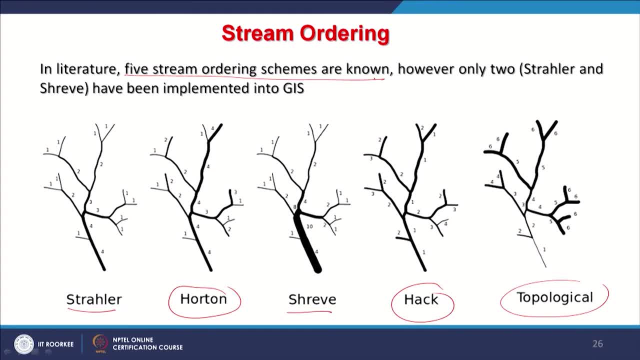 However, as I have mentioned that in softwares only either stellar or stream or both have been implemented- not many. Personally, my choice is for this stream method, which I find is very simple. After all, we have to give some order.